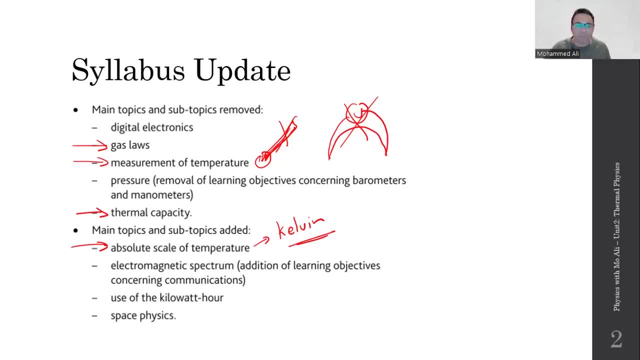 We'll discuss the difference between Kelvin and Celsius today, But I want to focus on this thing over here. The reason I'm saying they claim to have removed the term gas laws and why it's not really honest of them is because they removed the names of the laws. 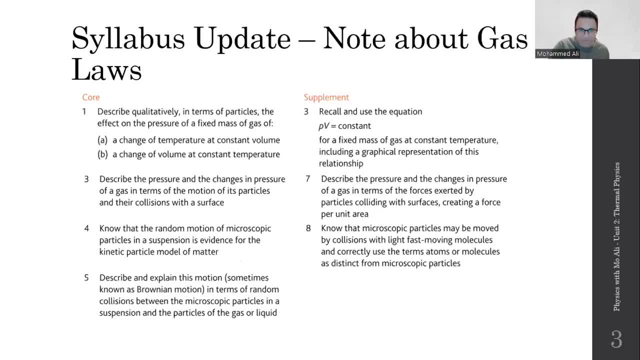 obviously, But let me show you something in the syllabus itself. This is the note about gas laws in the syllabus. This is the new syllabus. It asks you to describe the effect on pressure of a gas of changing temperature and changing volume, And then you calculate pressure and volume. 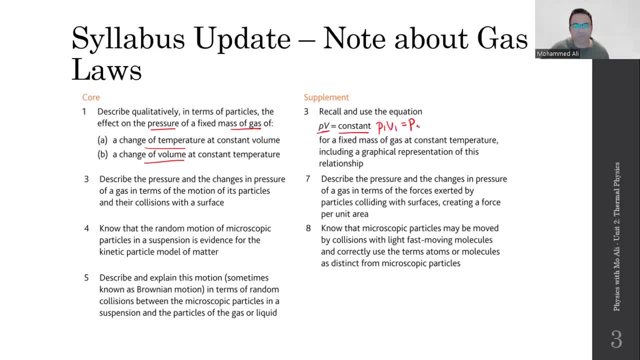 using PV equals constant or P1 V1 equals P2- V2.. If you've studied anything before this, you realize that this still exists. See, it's in the syllabus. They've claimed to have removed gas laws, but this is still there. So describing how the pressure and change in temperature 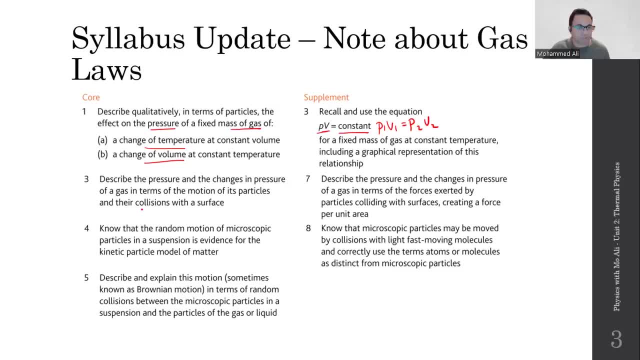 change in pressure of a gas in terms of the motion of the particles and collisions. that's still there, So still. gases describe the pressure and changes in pressure of a gas in terms of forces exerted by the particles colliding on the surface, creating pressure again that's. 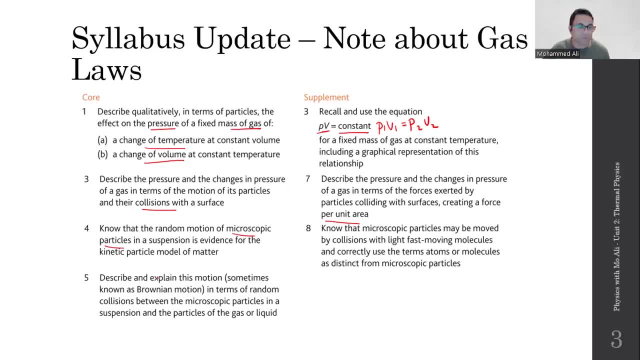 still there. Random motion of microscopic particles, which we also call Brownian motion, is still there. Knowing that microscopic particles may be moved by collisions with light, fast moving molecules and correctly use the terms Atoms or molecules, This is still related to Brownian motion and still there. So even 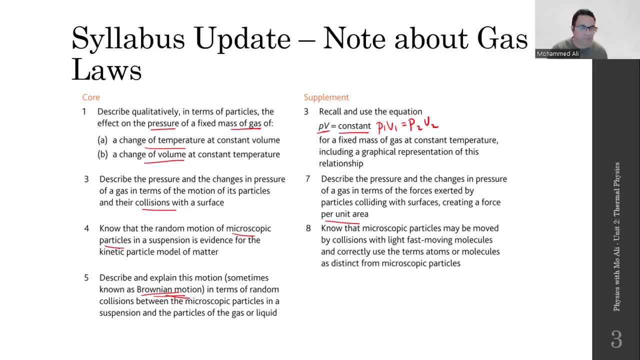 though the syllabus claims to have removed gas laws, whether you're a core student or whether you're an extended student- so extended on the right and core on the left- it really hasn't been removed, not directly, not the way you think it has been. So most of the 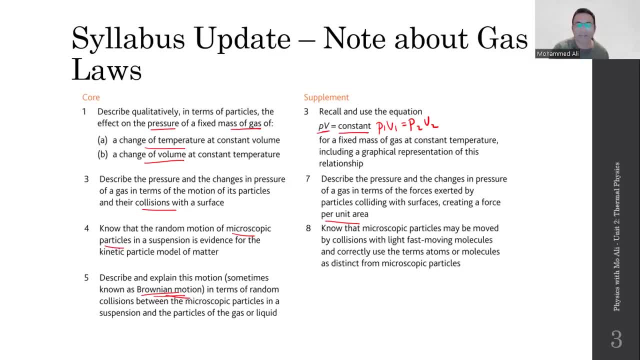 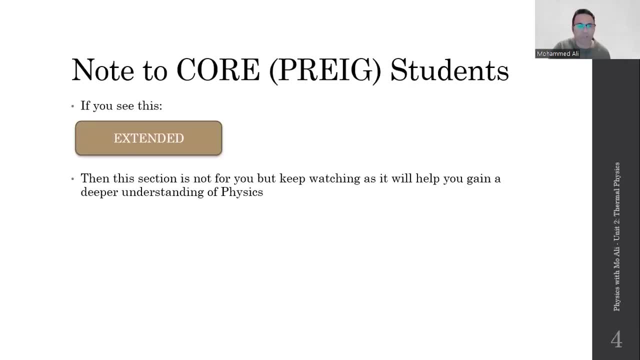 old questions in the past. papers that involve the behavior of gases will still work, So let them, just as they are. Keep going Right. Just a reminder note to course students: if you ever see a slide or a rule or an equation with the term extended on it, this is not. 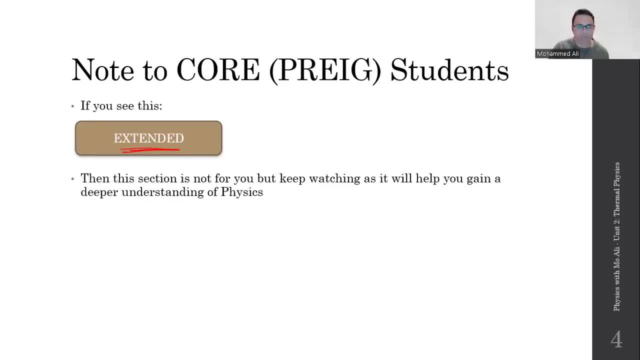 for you. It's not in your final exam, but listen to the chapter anyway. listen to the topic anyway. it will help develop your overall understanding of physics and it'll help you understand some of the concepts that you do study in core but we don't elaborate on. 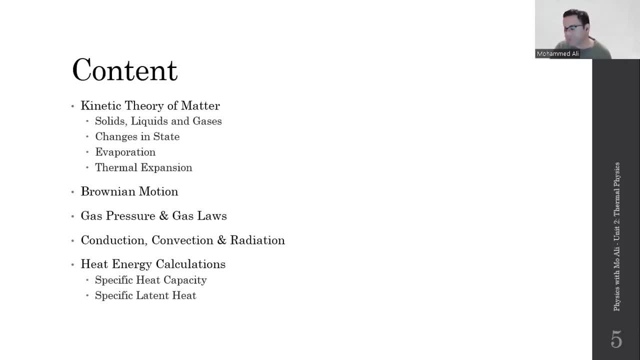 You get the idea. So what are we studying today? It's a very short unit. We'll talk about the kinetic theory of matter, meaning the difference between solids, liquids and gases. A lot of people complain It sounds a lot like chemistry, kind of does And what's. 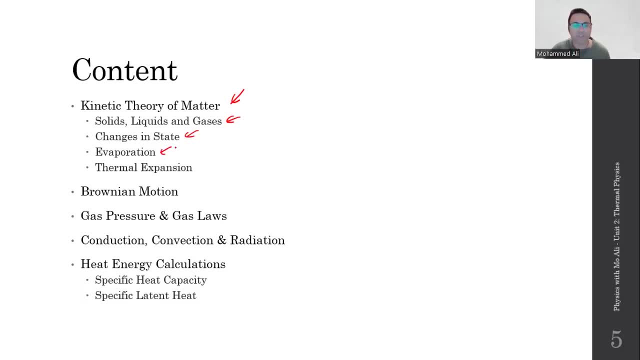 the change in state, melting and boiling and evaporation, and the details behind the change in state. We'll also talk about thermal expansion: change in what volume of a gas or a solid or a liquid when heated. Now, while we're talking about these, we're also going to be talking about the Kelvin. 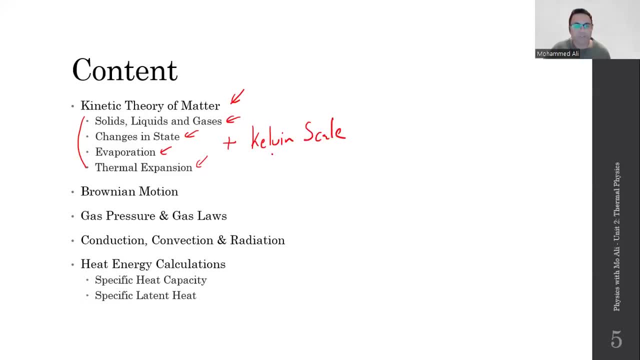 scale. So how do we measure temperature in Kelvin from Celsius? Once we define what temperature is, we'll talk about Brownian motion and the behavior of gases. Again, these have not changed, So I'm keeping them, as is conduction, convection, radiation, because these, these are the methods. 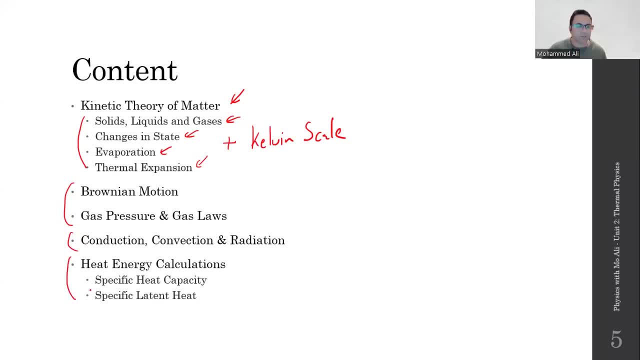 of heat transfer that we're familiar with, And we'll finalize by talking about how we calculate heat energy, whether it's the change in temperature of an object, using MC, Delta t, or change in state of an object, which is ml. Obviously, any course students listening to this right now don't Worry, This is extended. 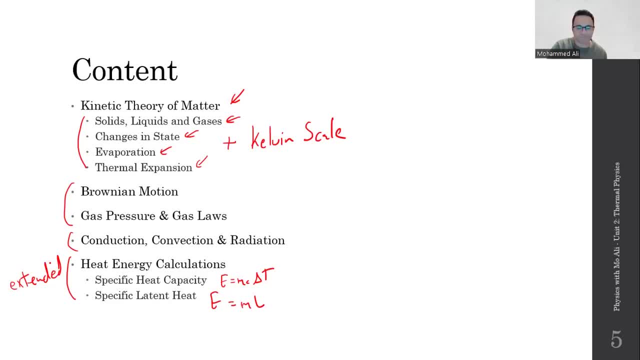 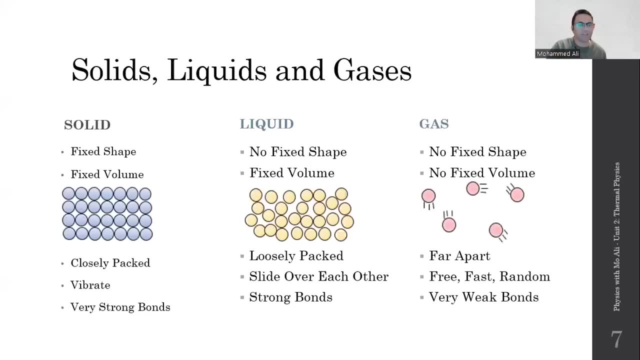 and you'll see that note as we move along. the slice song plays. Let's get started. solids, liquids and gases. the basics All matter consists of solids and liquids, and gases go to Shallow. miniature clip now of three, one of three states of matter, quite simple. but in unit two, when it comes to thermophysics, 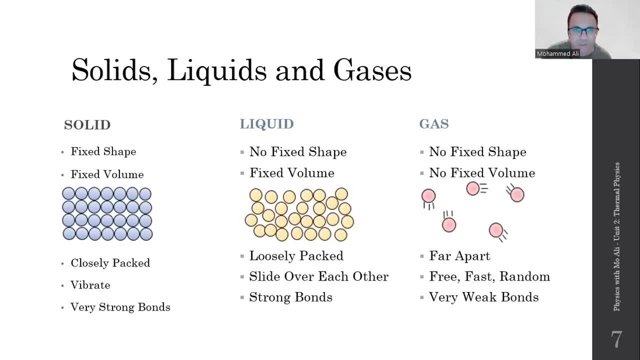 please keep in mind: when we describe something, any kind of matter, we often describe it twice: from the outside: what's going to, what's going on to it, what's happening to its shape, to its volume, to its mass, to its pressure? so we talk about the outer shape of the object and then we have to 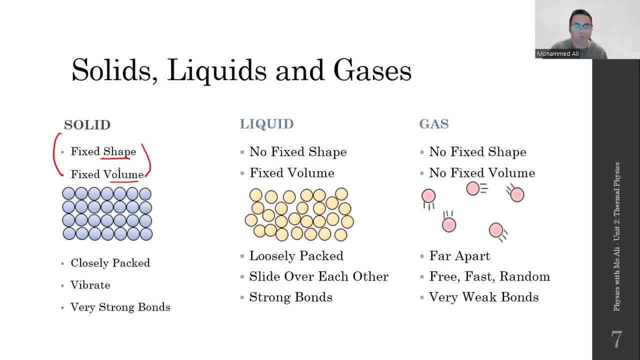 describe why that outer shape or volume or mass or pressure has been affected in terms of molecules. so all matter, just to simplify, will be assumed to be made up of molecules, and all of these molecules are either moving- they're vibrating, in place they have- or obviously sliding, moving freely. they also have a certain space between them. 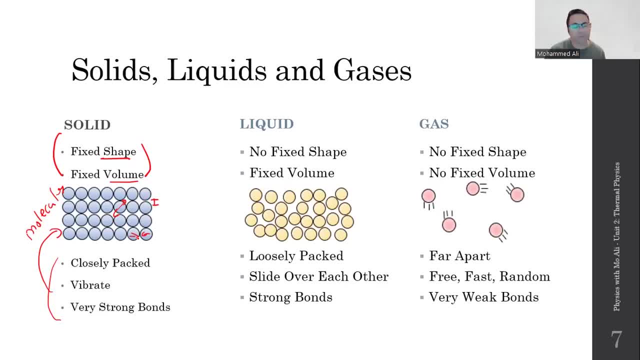 and they have attractive forces between them, which we will call intermolecular forces or simply bonds. james bond, i know it's an old joke, i'm never gonna let it go, never gonna give you up. i rickrolled you, sorry. let's move on. it's way too early for me to do this. 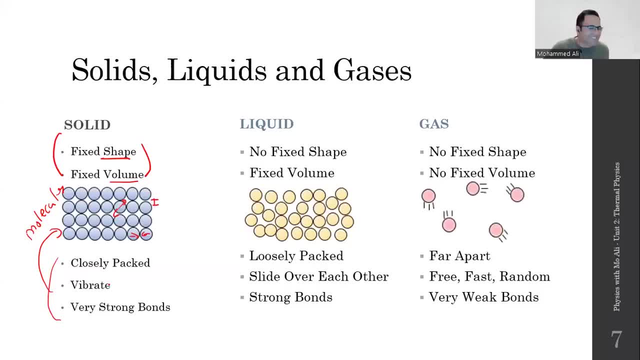 come on. so what was i saying? yes, so we're going to talk about any kind of matter in the rest of this unit twice, on the outside and on the inside. so on the outside, solids have a fixed shape and a fixed volume. inside, the molecules are closely. 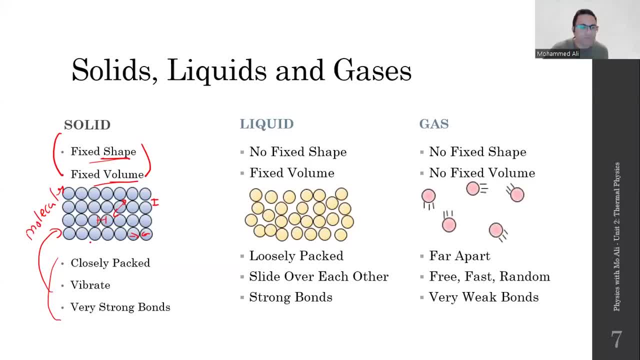 packed. they're very close to each other- very small spaces- and they vibrate about a fixed position. they don't move around freely and their bonds are very, very, very strong. liquids, on the other hand, have no fixed shape, but they do have a fixed volume. in other words, they take the volume. 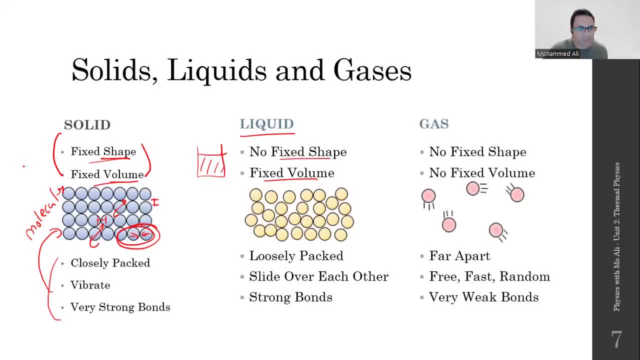 sorry, they take the shape of the container they're in solids have a nice fixed shape and that doesn't change. however, in terms of molecules, they're loosely packed, which means they have small spacing between the molecules and they slide over each other. finally, the bonds between them. 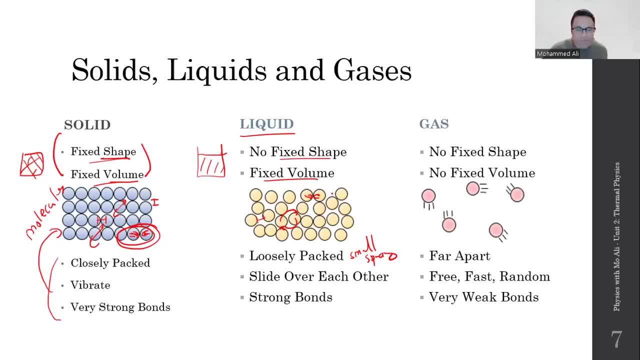 are still strong. they're not very strong like a solids, but they're strong. this is why they also have a fixed volume. it's thanks to the strength of these bonds, but they have a fixed volume. this has a fixed volume and a fixed shape because the bonds are. 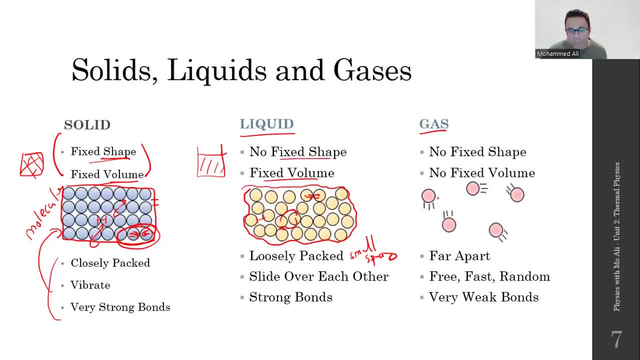 extremely strong gases, on the other hand, have no fixed shape and no fixed volume. why? because, in terms of molecules, first of all, they have very large spaces and they move very freely and fast, at high speeds and randomly, because they have very weak, or what we call virtually no bonds. so that's the difference. 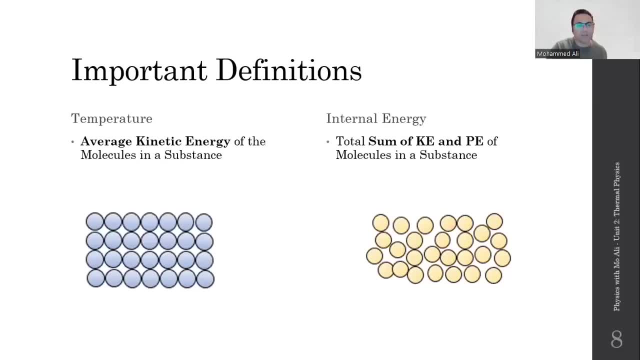 between them. next, we need to know how to define temperature. whenever you heat a substance, on the outside it gets hotter, the temperature rises, but on the inside the molecules gain energy and start to move. maybe it vibrates. if this is a solid, for example, they vibrate faster and the 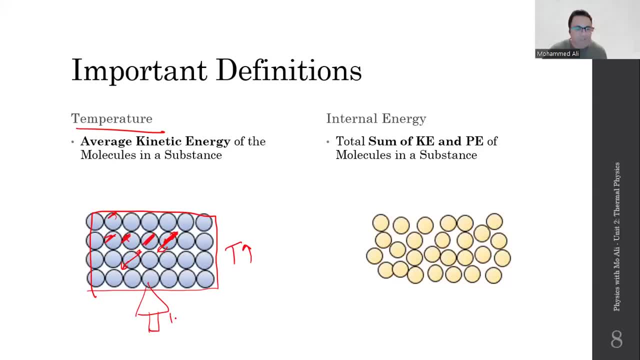 faster and faster and faster they vibrate, the higher the temperature of the substance. so when you heat something, the molecules inside move faster. this is why we define temperature as the average kinetic energy of the molecules in a substance. it's often measured in degrees Celsius. basically, how fast are the molecules moving? heat it up- molecules- move faster. cool it down- molecules. 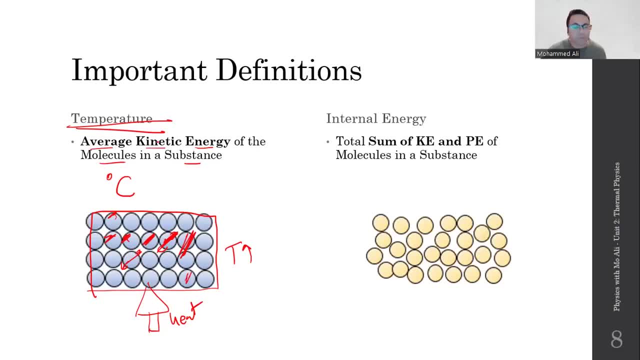 move slower. but now that we've mentioned that molecules have kinetic energy- molecules inside a substance, they also have potential energy, like they have both kinetic because they're moving and they have potential because they're trying to attract each other the further away the molecules are from each 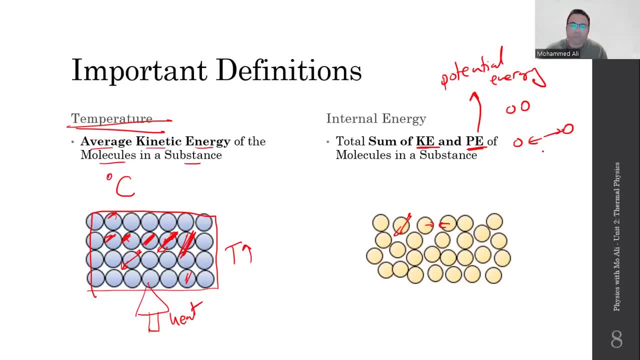 other, the more potential energy they have. and the closer the molecules are to each other, the less potential energy they have. so potential energy of the molecules depends on their spacing, at least until we hit a gas. but I'm not going to get into details about gases, right? 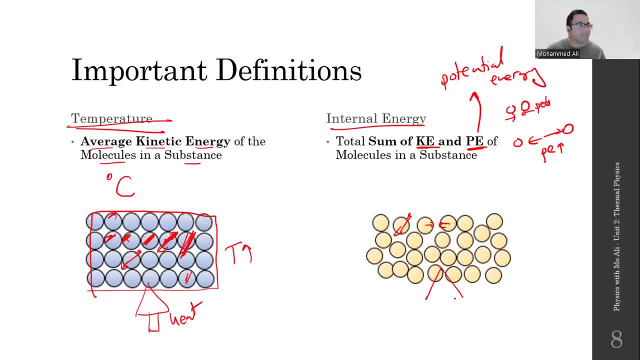 this is what we call internal energy. so when you heat something, the internal energy of that gas or solid or liquid increases because the molecules inside move faster and they also move farther apart. we are going to segue this into thermal expansion later. yeah, let's talk about temperature scale. 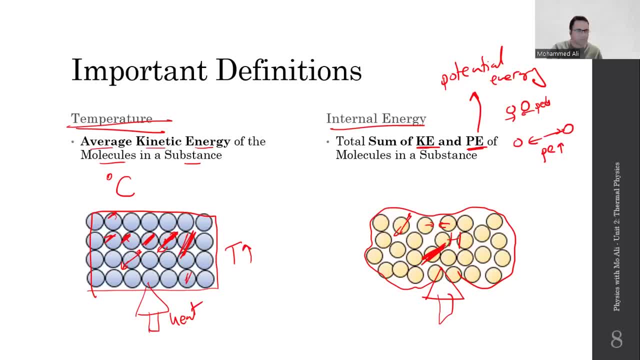 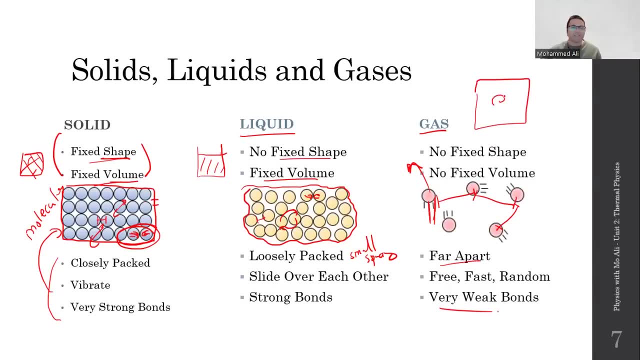 but before that actually there's a question, and it's actually relevant to the previous part. what do you mean by no fixed volume? a gas has no fixed shape and no fixed volume, meaning a gas fills up whatever container it's in. so if I ask you what's the size of this gas, it's the size of the container. 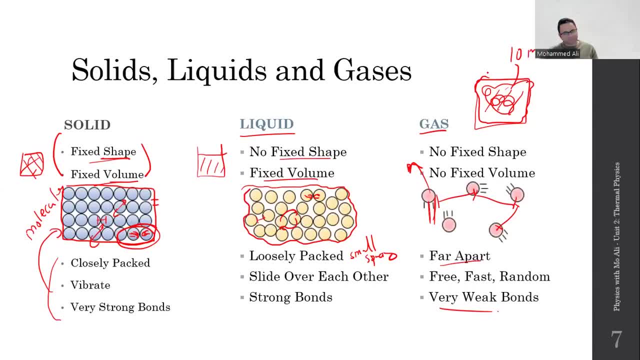 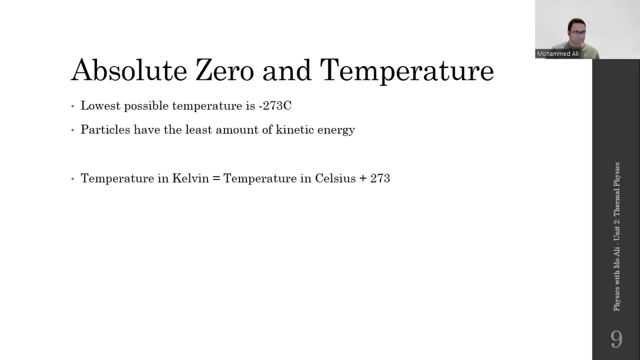 if I tell you the container is 10 meter square, a cubed I mean, then the gas inside is also 10 meter cubed. it takes the shape and the volume of the container. yeah, let's talk about the Kelvin scale. let's talk about the Kelvin scale. 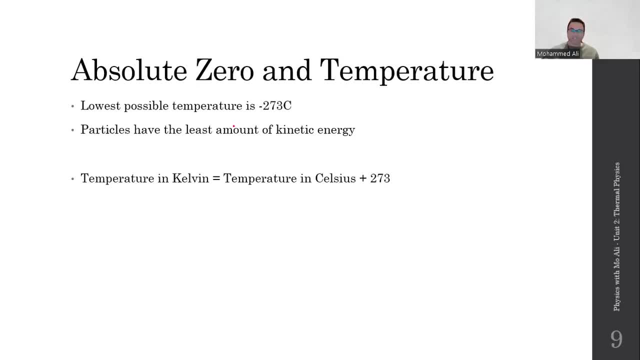 now let me identify a problem with the Celsius scale before we talk about the Kelvin scale. the problem with the Celsius scale is that it has negative values. the smallest value on the Celsius scale is not zero. zero is the melting point of ice, whereas 100 is the boiling point of water. 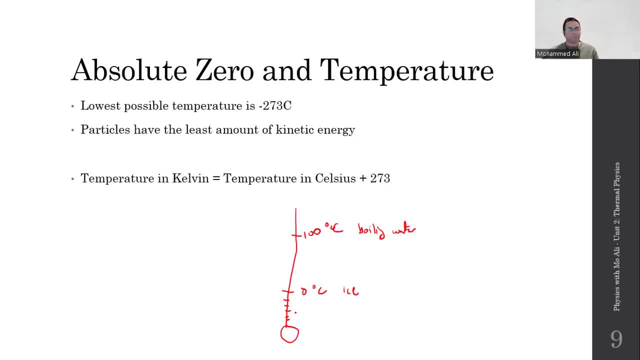 which means there is stuff that's colder than ice, which makes sense. you have temperatures like negative 10, negative 20, negative 50 and so on. so gets colder and colder and colder. but here's the thing: what was the definition of temperature? if you remember, it was defined as the average kinetic. 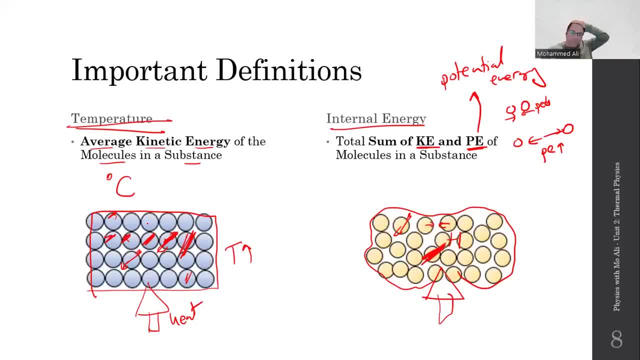 energy of the molecules in a substance. why? because it depends on how fast the molecules are moving speed. average kinetic energy is because we're getting the average speed. we're not looking at the fastest, we're not looking at the slowest, we're looking at something in between. so the higher, the 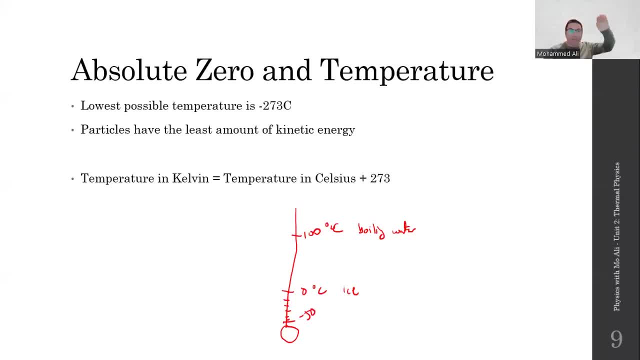 temperature of substance, the faster the molecules should move, and the lower the temperature of a substance, the slower the molecules should move and, technically speaking, at zero degrees of whatever this unit is. this should mean that the molecules have zero kinetic energy, which is false when it comes to the celsius scale, because there's stuff that's colder than zero now. kelvin, lord kelvin. 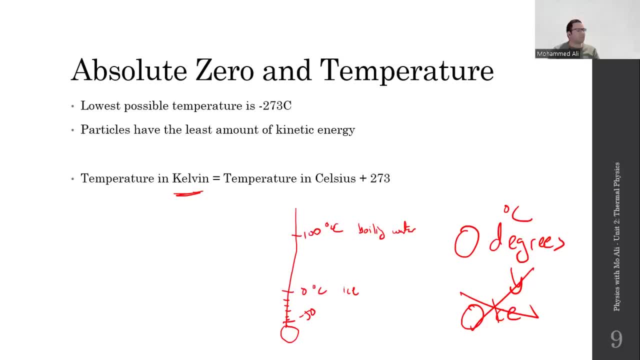 did not like that idea a very long time ago. so he decided to find out the coldest temperature in the universe so he can change the scale a bit. through his mathematics and experimentation he discovered that the coldest temperature you can ever reach is negative 273.15. but we just ignore. 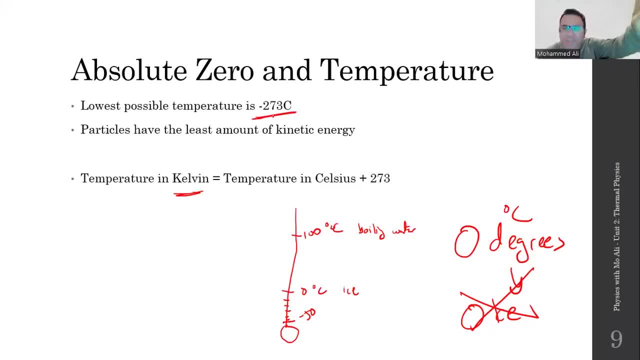 that the decimals degree celsius. that's the coldest temperature in the universe. this is the temperature at which the molecules have no kinetic energy or the least amount of kinetic energy. the molecules of a substance are not moving. molecules of substance are not a moving. so he put down a scale next to the original celsius scale and he put his zero where the coldest. 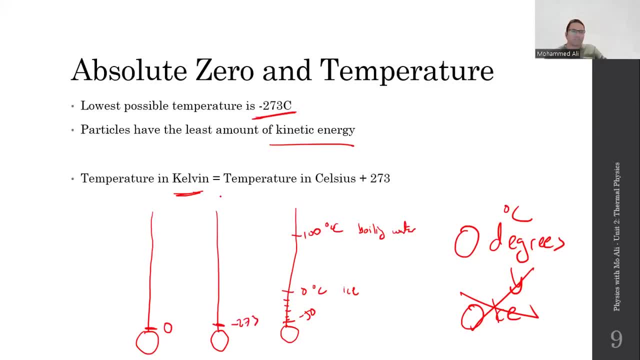 celsius degree is. so this is in degrees celsius, at negative 273. this is kelvin's zero and he used the exact same scale. so he jumped up the same number of degrees so that the zero is 273 degrees. the hundred celsius is 373 degrees. so you're moving the same number of degrees, so it's almost. 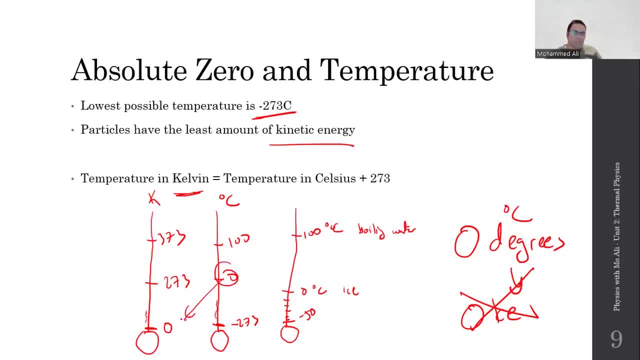 the same scale. it's just that we shifted where the zero is and we call this absolute zero. we call this absolute zero. it's very easy to convert kelvin to celsius or back. kelvin is celsius plus 273. so if i say 100 celsius, that's to 373 kelvin, because you add 273. 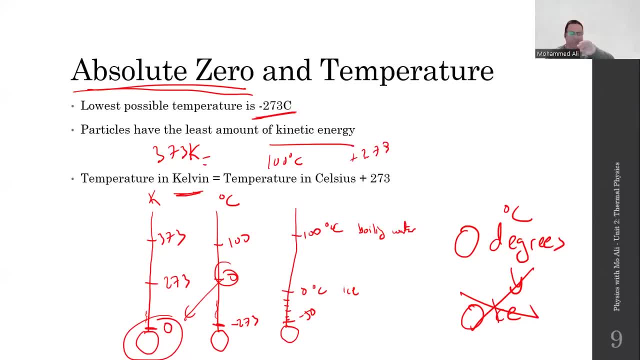 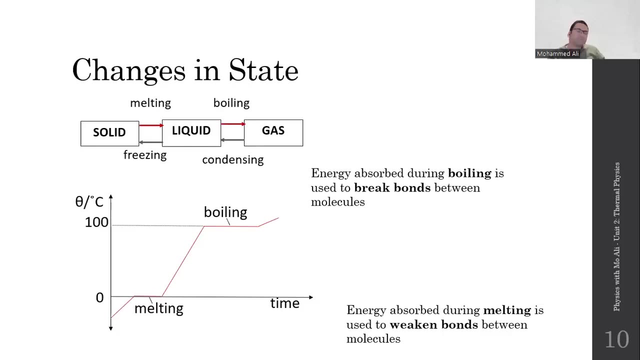 obviously you do the reverse. if you're changing celsius to a sorry kelvin's celsius, you subtract 273. very good, now let's talk about how do we change states when you heat any kind of substance, a solid or liquid or gas. when you heat it, the temperature, 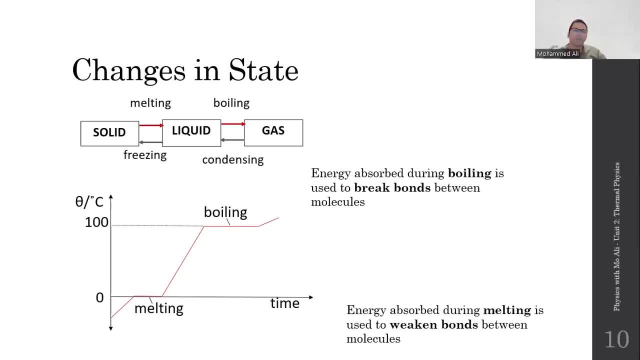 rises because the molecules are now moving faster and faster and faster. but once it reaches a certain temperature- let's say you start off as a solid with some ice, at negative 20 degrees or something- once it reaches the melting point, which is zero degrees celsius, that's the temperature. 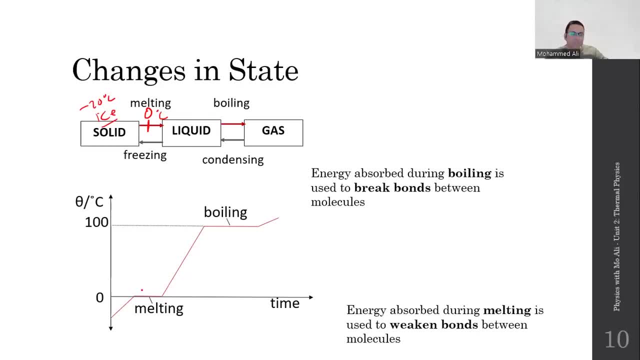 where ice starts to melt, it changes from solid to liquid and during melting the temperature stays constant. it doesn't change, does not change, which should make no sense. but then, once it's completed its process of melting and now the substance is a liquid, it gets hotter, it's no. 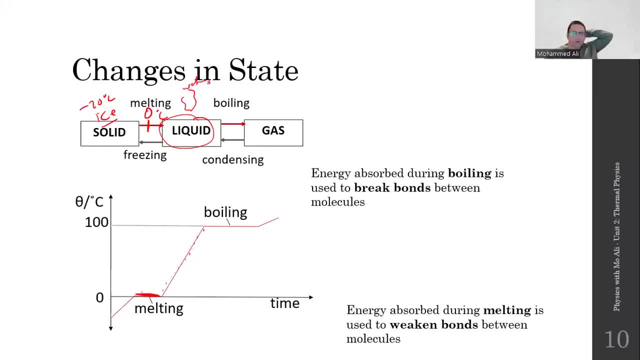 problem if you heat it up. this water is now hot. it's in liquid state, but once it reaches the boiling point, which is 100 degrees celsius, you'll find that the temperature stays constant again during the boiling process. during the boiling process, temperature stays constant until it's completely turned into a gas, and then the 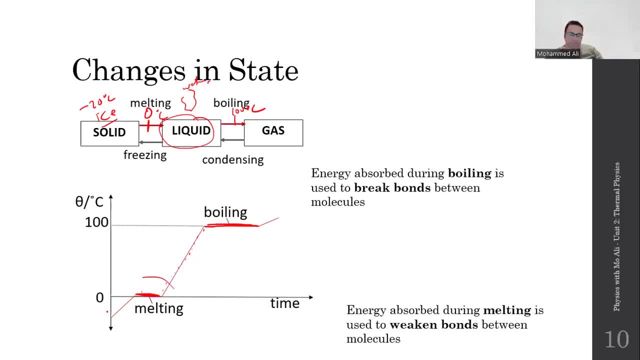 gas heats up. but the question is- and this is the most important question here- why is the temperature constant during melting and boiling? because naturally, when you heat a substance, the molecules inside want to move faster. so they do. but they also move farther apart, up to the limit of the bonds between them, like some molecules are. 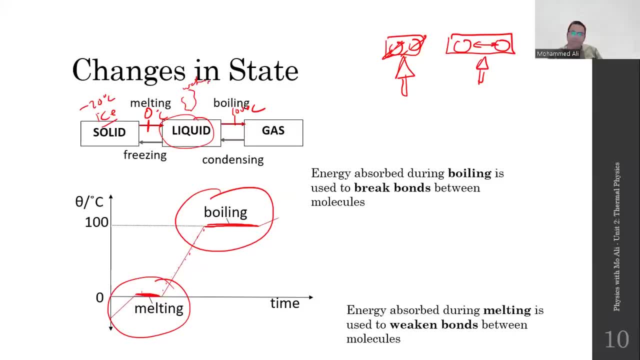 strongly bonded. but if you heat it up enough, what's going to happen? it can't move any further or any faster. so the kinetic energy of the substance does not increase during melting. instead, the energy is used to weaken the bonds between the molecules in order to push them farther apart, makes them weaker. 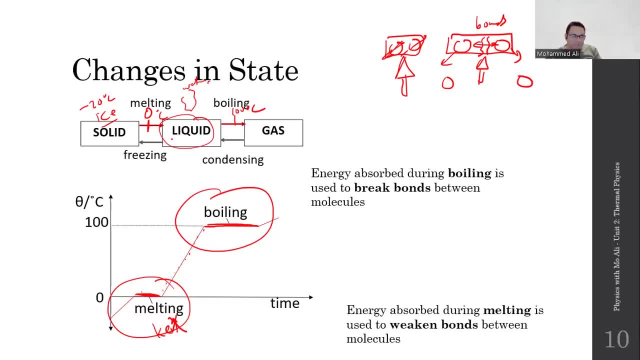 this is why the bonds in a solid are very strong, whereas in liquids we just say they're strong. what about boiling? well, if you leave the substance boil, some water to boil, it gets converted completely into a gas, because all of the energy is used to what, or a lot of the 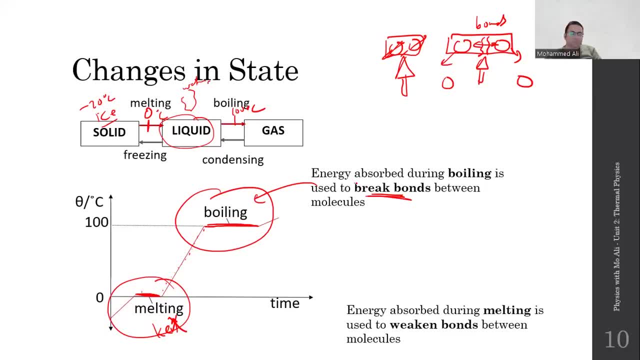 energy is to break the bonds between the molecules so they can successfully escape. okay, so during melting the temperature stays constant because the energy is used to weaken the bonds. during boiling, the temperature stays constant because the energy absorbed is used to break the bonds and the kinetic energy does not increase in either of these cases. it does not. 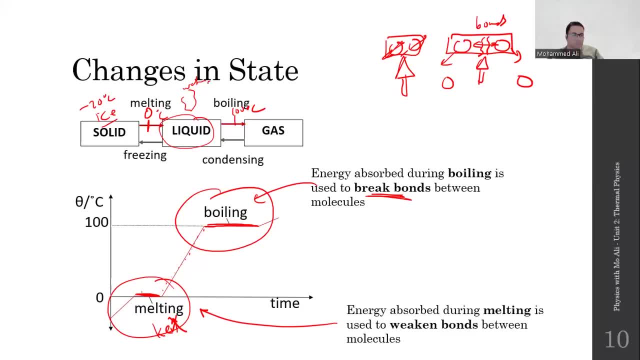 increase. so temperature is constant during melting and boiling. it's also constant during condensation and freezing. so if i draw this graph in reverse, during freezing and condensation the temperature also stays constant because the energy is used for something else, for the potential energy. so to answer the question, that's on the chat box here: 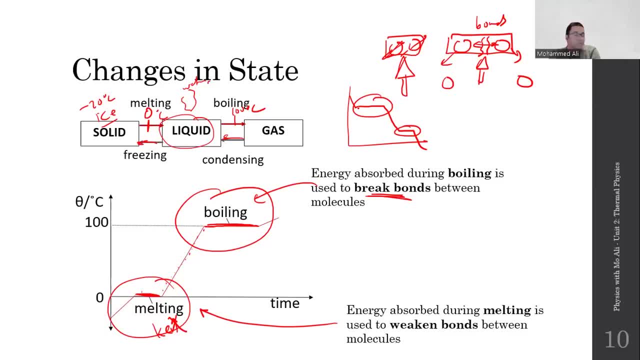 or in the chat box here. how do molecules have potential energy? because the molecules have space between them. if any two molecules are trying to attract each other but they're kept farther away from each other for reasons, whatever the reasons are, they have potential energy because they're trying to attract each other for reasons. whatever the reasons are, they have potential energy. 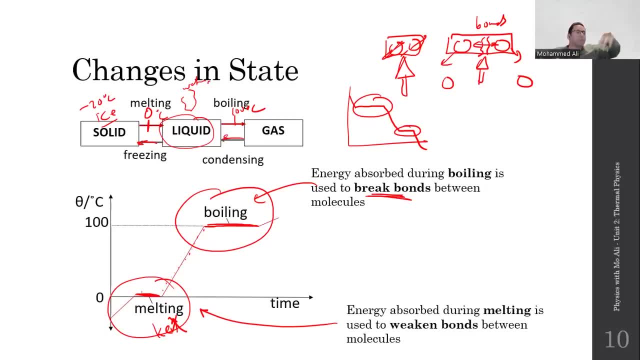 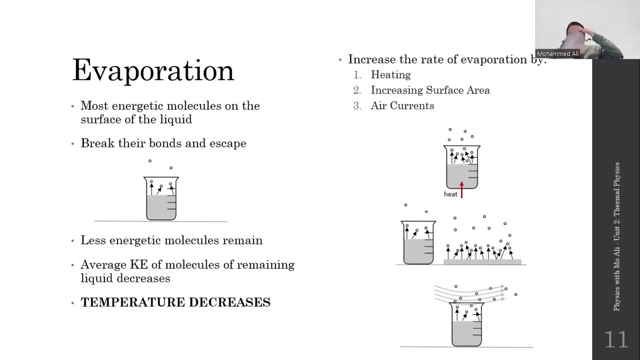 and the farther and farther and farther the molecules are from each other, the more potential energy these molecules have. okay, very good. next up, one more change in state is called evaporation. what is evaporation? it's when the most energetic molecules on the surface of a liquid break their bonds and escape, so when 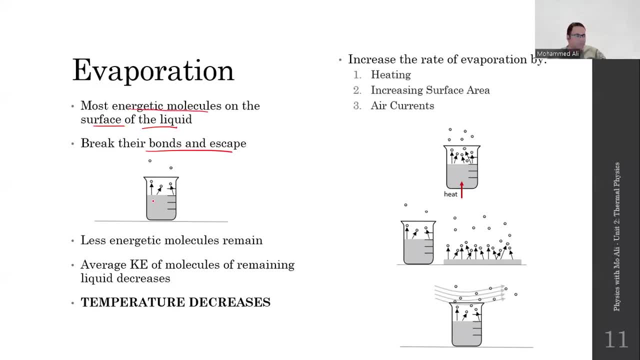 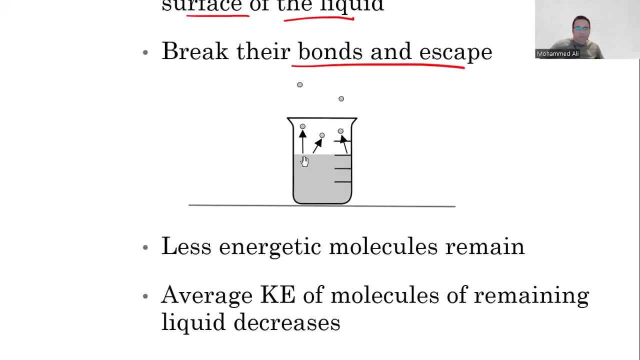 a liquid evaporates. it doesn't just evaporate because, hey, it's just just wants to. it's because, if you remember, we defined temperature as the average kinetic energy. that's because some molecules have very like. if we take a look here, some molecules have very high temperatures and energies and some molecules have less energy. temperature is a. 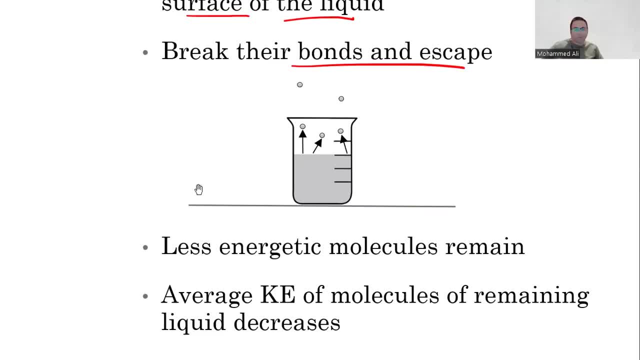 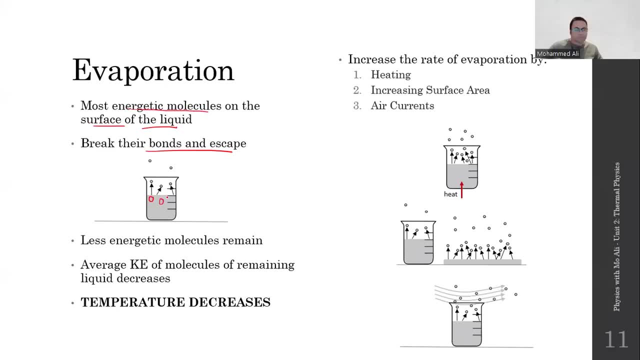 measure of their average. but if you have the most energetic molecules, if you have the most energetic molecules, people already on the surface of the liquid, meaning they have most of the energy of the substance. what do they do that energy? they break their bonds and they escape. so now the liquid has changed into a 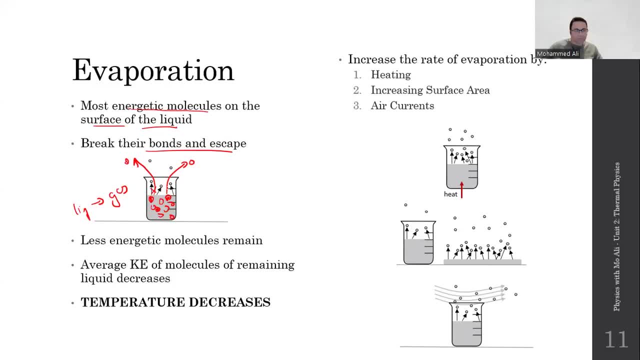 gas. a liquid has changed the gas. you've broken your bonds in the escape without heating, like we have not heated the substance at all. this is just naturally on its own. but do you know what the problem with evaporation is? is that the more a substance evaporates and 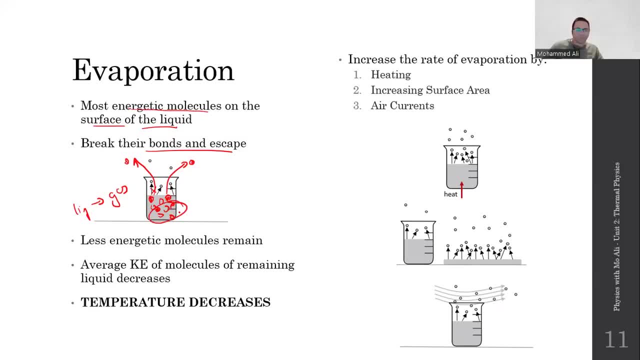 more and more energetic molecules leave. whatever is left behind has now less energy. so it has less energy than usual, less kinetic energy than usual. the temperature of the liquid decrease. this is why if you go take a shower and you get out of the shower, just wash your face or 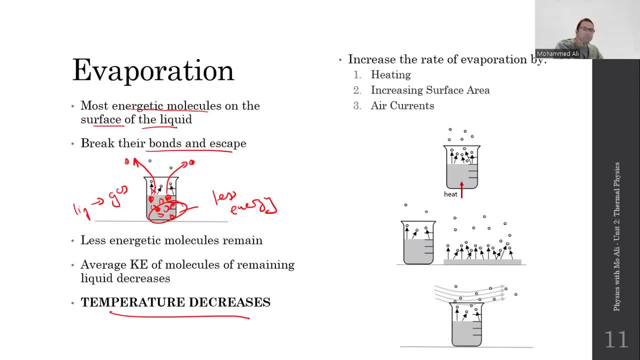 dump some water on your hair and just leave it there, you start to feel cold. why? because, as the liquid on your body evaporates and turns into a gas, it gets colder. the liquid itself gets colder. if the liquid gets colder, what will it do? it'll absorb heat from whatever is stuck to it. so this is why we sweat, by the way, like the reason. 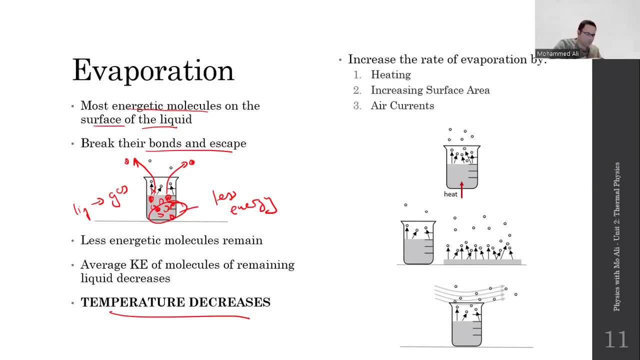 we sweat is because sweat, after it gets released, is on all over your skin, all over your body, and it's trying to escape. it's evaporating. but as the sweat evaporates, the temperature of the remaining sweat decreases, so it absorbs heat from your body to continue evaporating and you cool down. 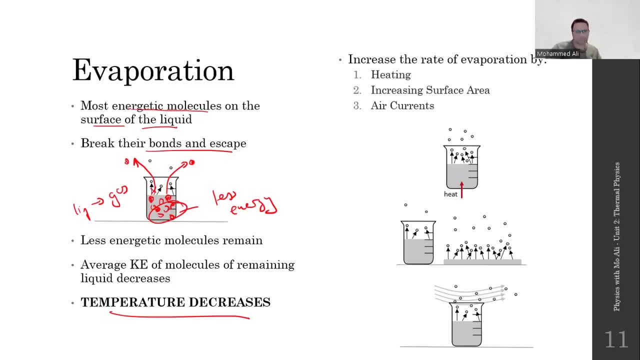 so the temperature decreases. there are three things that we can do to increase the rate of evaporation. you can heat it. obviously that's more energy. you can increase the surface area, so just dump this water onto the floor and since evaporation is so important, you can heat it. obviously that's more energy you can increase. 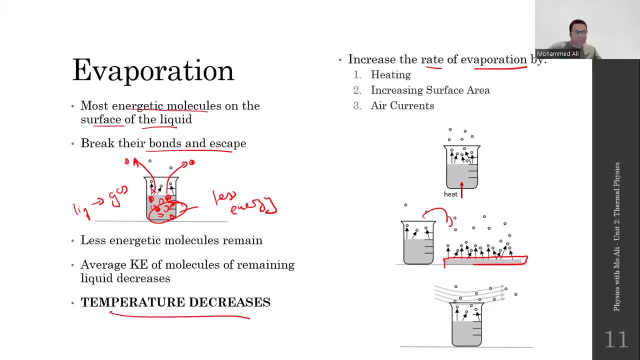 the surface area. you can heat it. obviously that's more energy. you can heat it, obviously that's more energy. evaporation only happens to the most energetic molecules on the surface. the more surface area i have, the better. increasing the surface area and finally, air currents, like if i've got some wind. 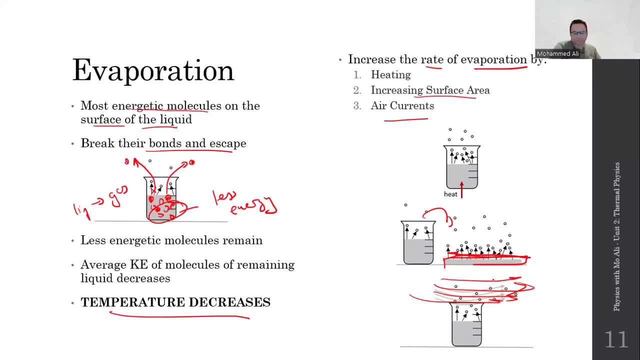 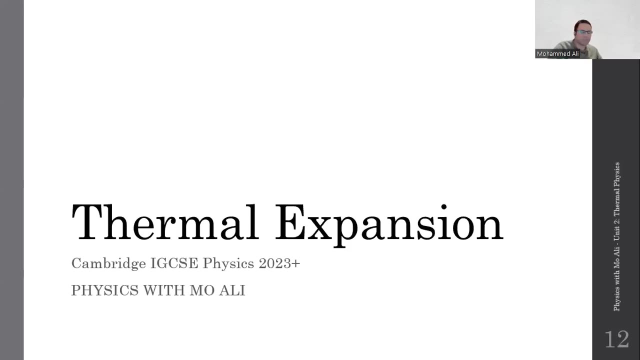 like if i have a fan running or just got some wind, a breeze passing by. what does that breeze do? it gives energy to the molecules on the surface, so these molecules can now escape faster. that is before i move on to thermal expansion. any questions about the previous section: solids and liquids and gases. 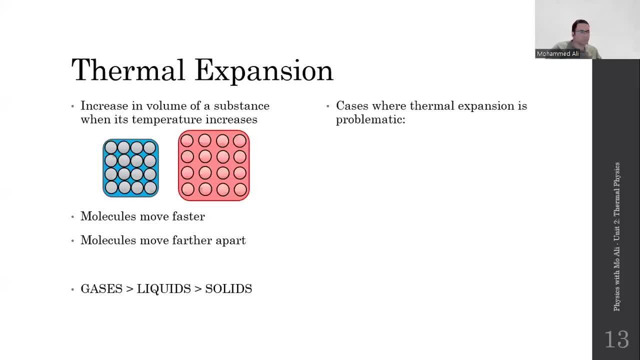 no, okay, very good, let's talk about thermal expansion. what is it? we've already mentioned it before, by the way, but when you heat something, when you heat the substance- a solid or liquid or gas- the volume increases. why? because, as we said, when you heat something the molecules move faster, but then they also move further apart. 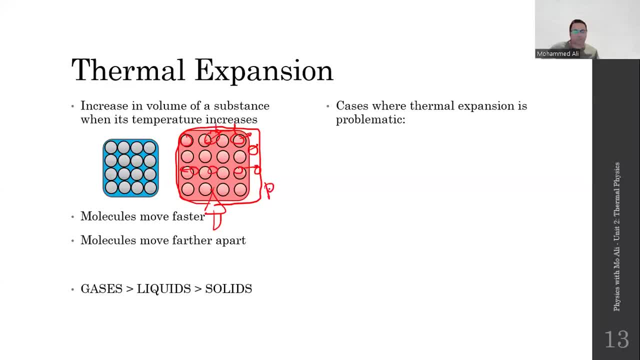 so as the space between the molecules increases, the pressure increases. okay, i'm sorry, not the pressure. what was i saying? not the pressure? the volume increases my bad volume volume. i need to ventilate this room. i'm lacking looks. so do all substances expand the same? i would say no. 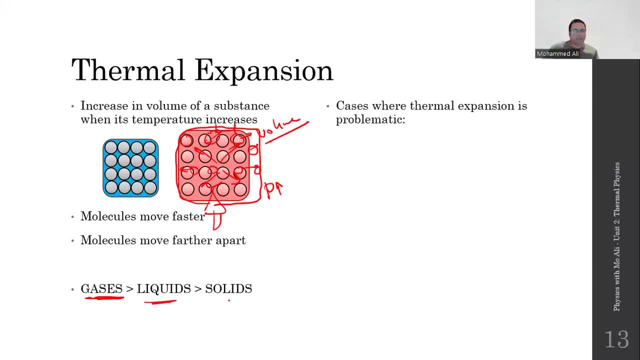 gases expand more than liquids and liquids expand more than solids. gases expand more than liquids and liquids expand more than solids. why? because gases are already far apart and they have very weak bonds. liquids are closer to each other with stronger bonds and solids already have superimposed. 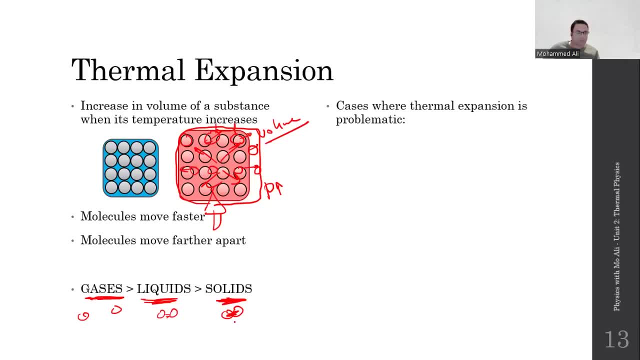 more than solids, and liquids are already stronger than solids, and solids are already stronger than already super close with a very strong bond. so it's hard to make these molecules move farther apart. it's much easier to make a gas molecule move farther away from other gas molecules. 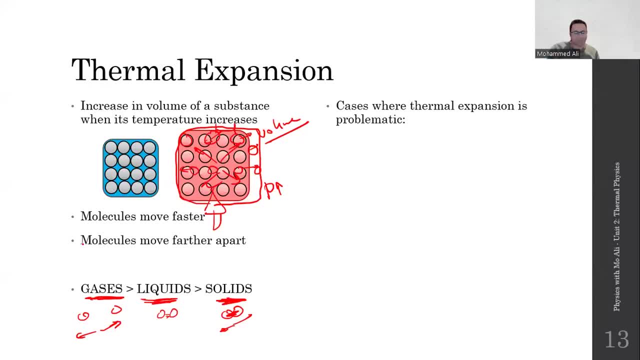 now, obviously thermal expansion depends on the temperature. heat it more, it expands more clearly. and thermal expansion also depends on the initial size of the object. meaning if you haven't had an object that's very small and you have another object that's a lot longer and you heat them both the same temperature, they will both expand, but the longer object. 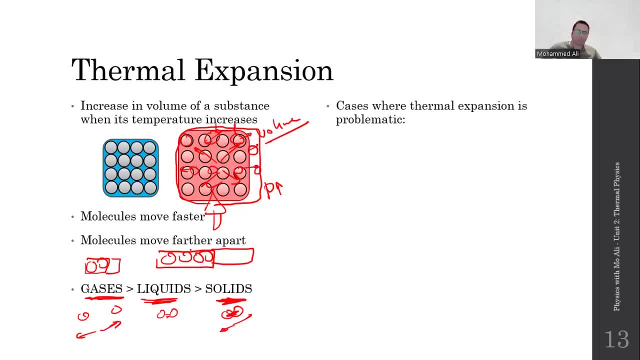 will expand more than the shorter object simply because it's got more matter and molecules to move farther away from it. good, you cases where thermal expansion is a problem. so where is it problematic? well, let's mention a couple of examples. so you probably remember the railway tracks, right railway tracks, if you have. 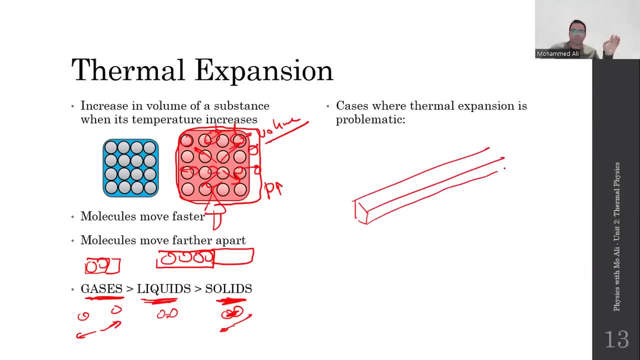 a railway track like this and you just let it expand. over time it will expand, but it won't expand the way you want because it's held in place with nails and screws and everything else. it ends up buckling, meaning it just bends all over itself like this. 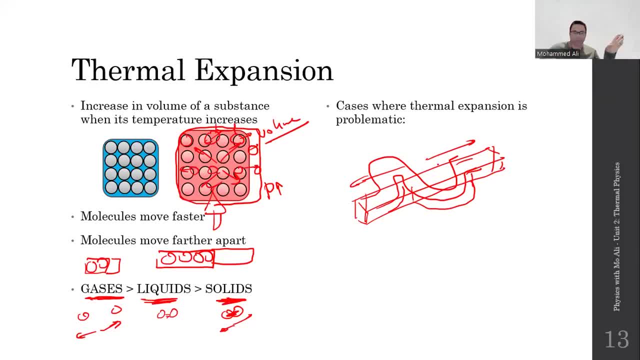 and any train that tries to go over this will derail for sure. so how do we fix this? because it wants to get longer, so it can, so it gets longer from the sides. we always build our railway tracks within sections. why? because leaving sections allows each small section to expand a little bit when it gets hot. 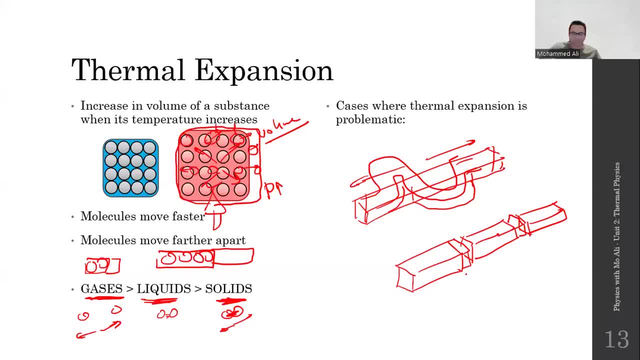 during the summer and during the winter it contracts and it goes back to its original size. it's not a problem. or even if it's slightly smaller, it will not matter at all. okay now, another problem with thermal expansion is that it's not going to expand over time. 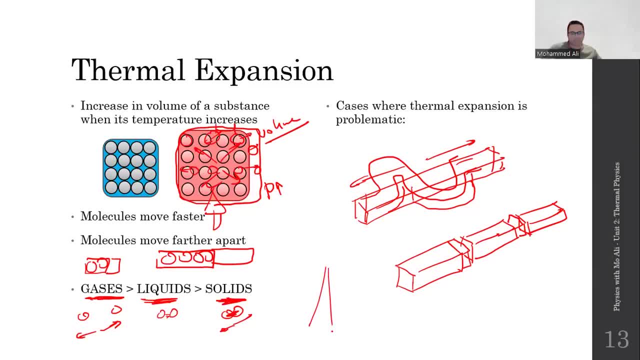 it's not going to expand over time. it's not going to expand over time. it's going to expand over time. it's going to expand over time and, honestly, it's more about thermal contraction than expansion. would be electrical cables, pylons, the reason why we hang electrical cables from these towers, or 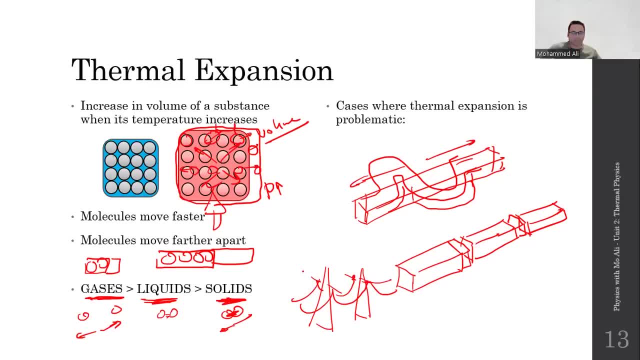 pylons and we hang them loose like this. we don't just stretch the pylons and stretch the wires in the air. get them why? because if you stretch it like this and it's not going to expand over time, it's not thermal expansion this time. that's the problem, it's contraction. 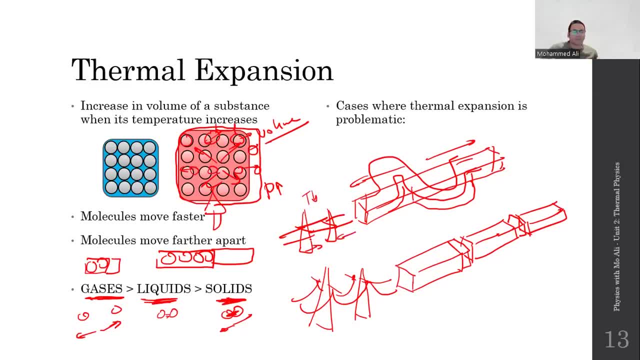 if it cools down, this cable will want to contract. it wants to get shorter and as it gets shorter it pulls on the towers, it pulls on the towers and it could break. but if you already give it some extra slack and then come winter when the temperature decreases and it wants to contract, it's still got. 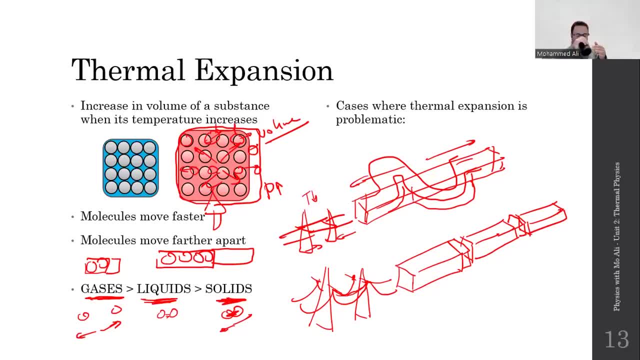 space to contract. so I don't think it's going to expand over time. so I don't think it's going to expand over time. so I don't think it's going to expand over time. uh, why is it longer? I'm sorry, why does it? here's a question, guys: why does it expand more when an object is longer? because 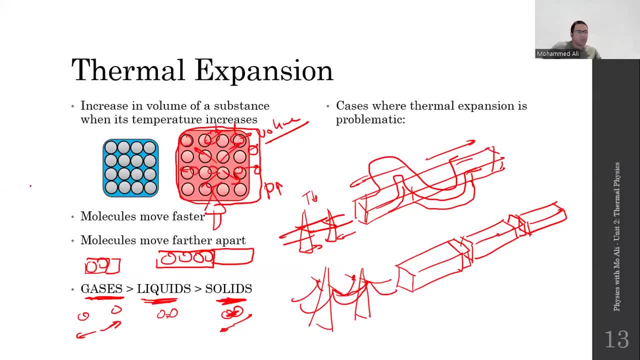 where does the expansion come from? the space between the molecules. if you only have two molecules and they move farther apart this way, this much here's your expansion. but if you had four molecules and they all expand with the same extra distance, this much, what's the total expansion? a lot more, even if you heat at the same temperature, which? 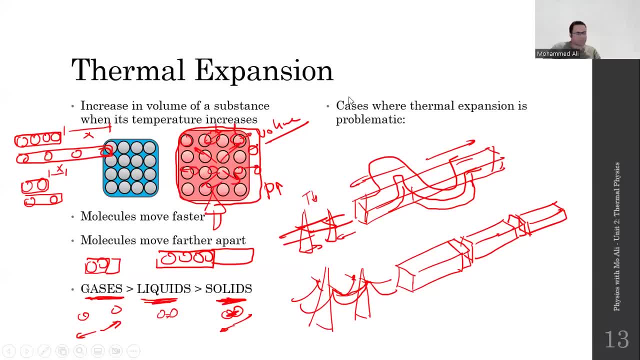 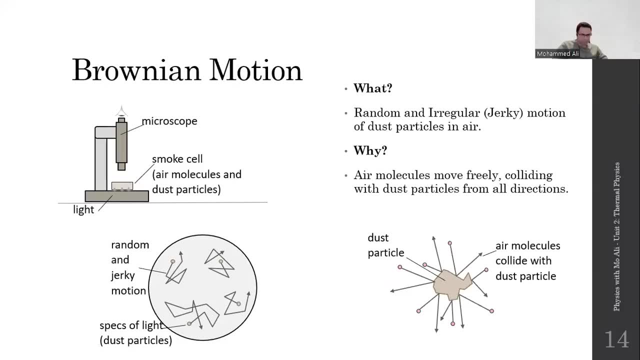 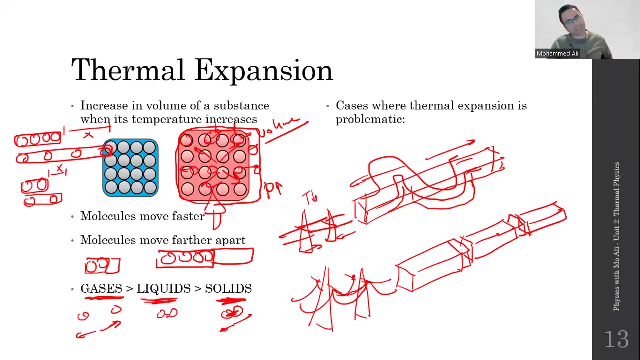 will increase. the space is the same. because you have more molecules, they'll expand more. now let's move on to the behavior of gases for a bit. let's talk about the Brownian motion, is it? I'm sorry, let's go back for a second. of course it's related to liquid expansion. I mean, when heated, what will happen to the? 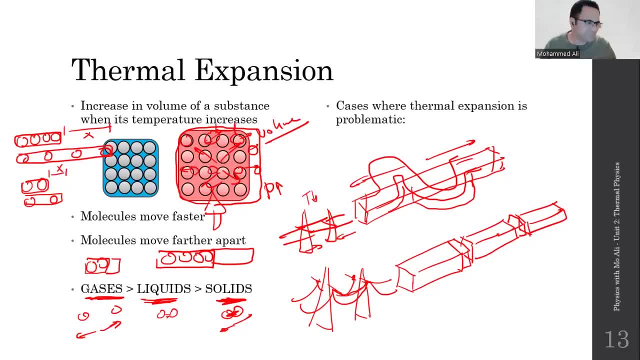 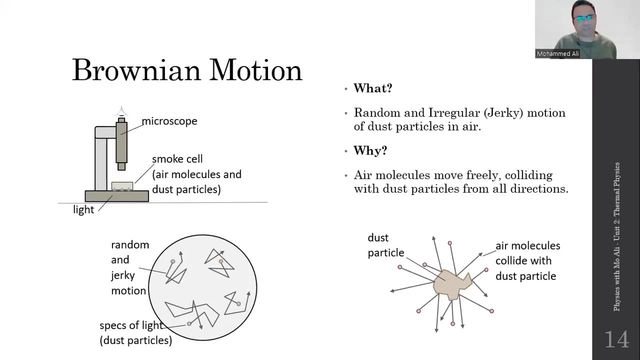 volume of a liquid. it will increase. it will expand right, because the space between the liquid molecules increase. that's all you need to know. so what's Brownian motion? or like Brownian motion as something people like to say, but Brownian is the correct term. so what's Brownian motion, Brownian motion? 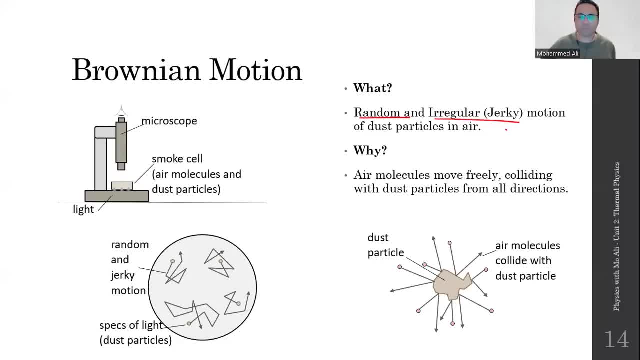 is defined as the random and jerky or irregular motion of dust particles in air. so if you look through a microscope into a smoke cell which got, which is a lot of dust and air molecules, obviously you will find that these small dust cells are moving random and 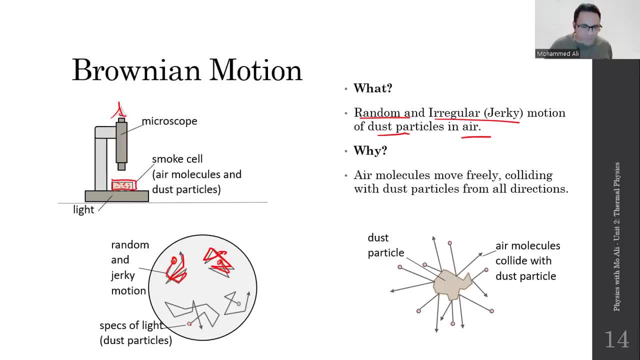 jerky like these small dust particles. we often call them specks of light, because the way microscopes work is that they shine a very strong light into whatever's inside- in this case it's smoke- so a lot of particles, and that light reflects up into the microscope's lenses and 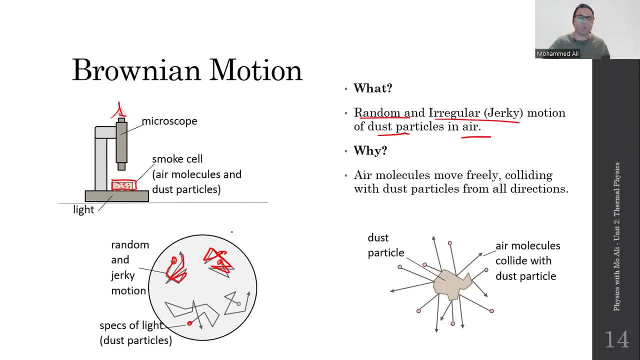 you see bright dots. why are they moving random and jerky? because the air molecules that are around them, as they're moving, they're also moving fast and randomly. but what do they do? they eventually collide with this dust particle. because they're moving randomly and jerky because they're moving. 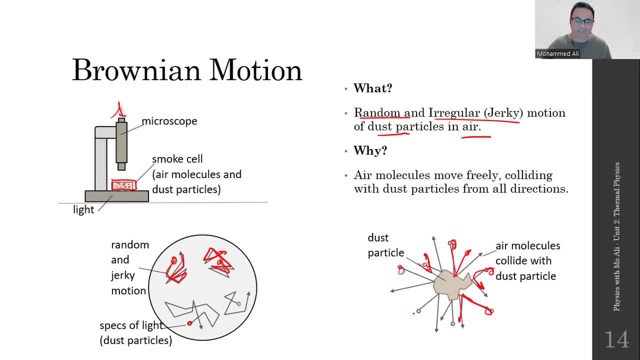 over millions of air molecules. but as these air molecules collide with the dust, this dust will move. think of it this way: you're slapping around the dust, the dust will move, and then, when it collides with new air molecules, it moves again, collides with new air molecules. 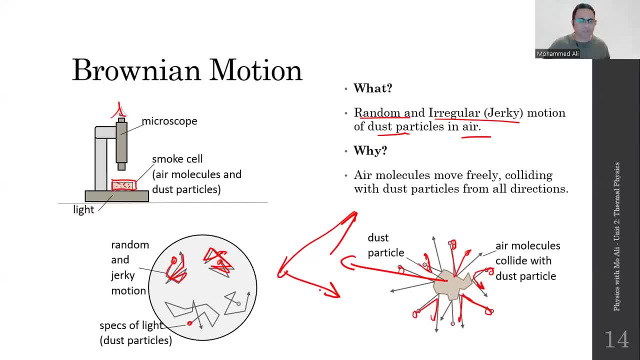 it moves again, collides with new or air molecules, moves again. that's why we call it jerky or irregular motion. it doesn't smoothly move around, no, no, no. it just gets further away from there, knocked away, because of the air molecules collide with it from all directions. this 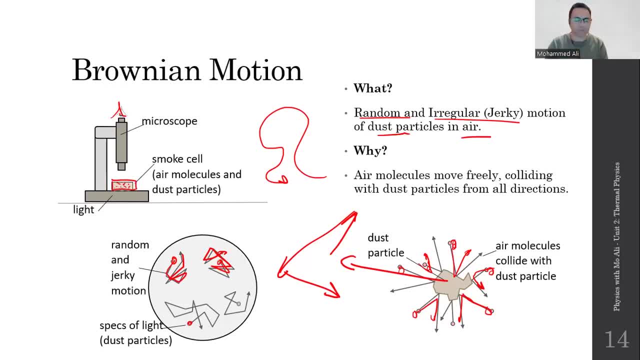 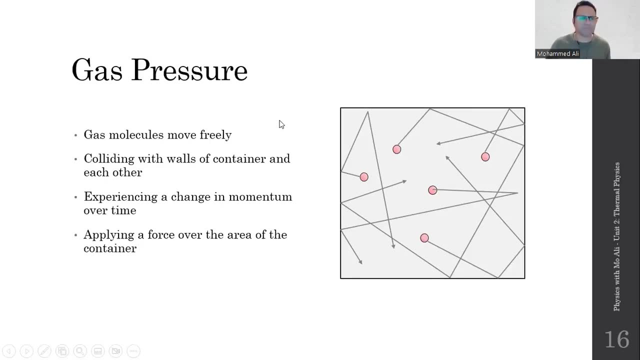 this row. this movement is called brownian motion, random jerky motion of dust particles in here. yeah, that slide came in a bit late, i don't know why. yeah, let's talk about the behavior of gas, like: how do gases behave? in order to understand how gases behave, we need to define how a gas 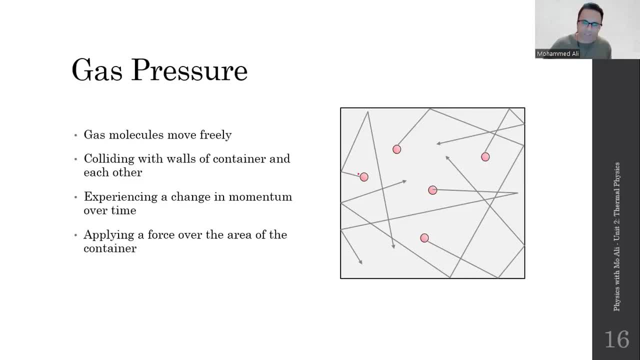 applies pressure. now take a look at a single molecule. as this gas is moving, it's colliding with the walls. every time a gas molecule collides with the walls, it experiences a change in momentum. it experiences a change in momentum because anything that collides with a wall for something and 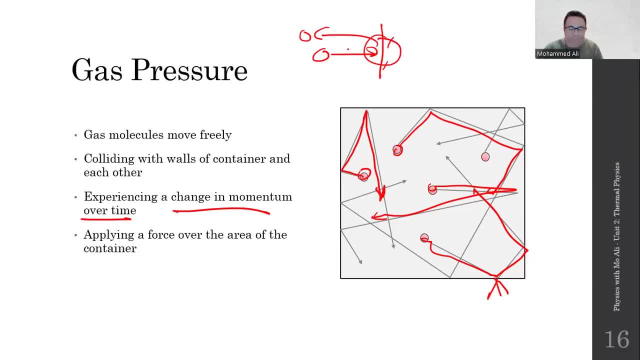 rebounds, experiences a change momentum here, because the direction has changed. maybe the speed has changed as well. now you may be saying, okay, so what? let it change? well, that collision and change momentum applies a force, and if you apply that force over a large area of whatever this container is, this will give you pressure. 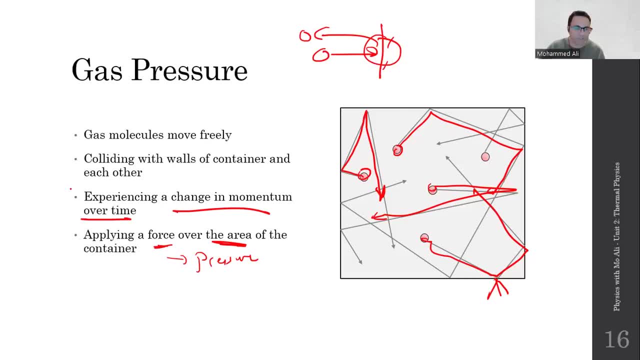 so this is just something that you can just see and that's the way it will change now. any mention of momentum, just just a second like: see this: here, this small part is extended, so i'm not going to be mentioning change in momentum or anything else. when it comes to core, 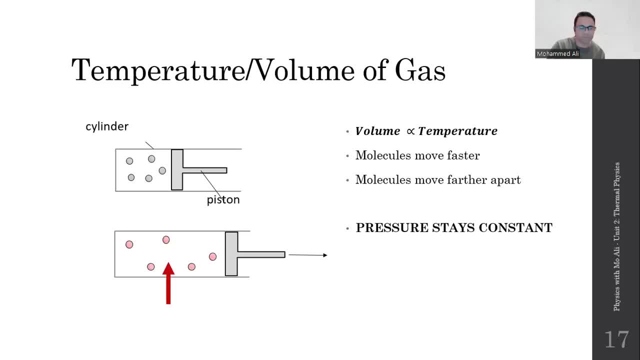 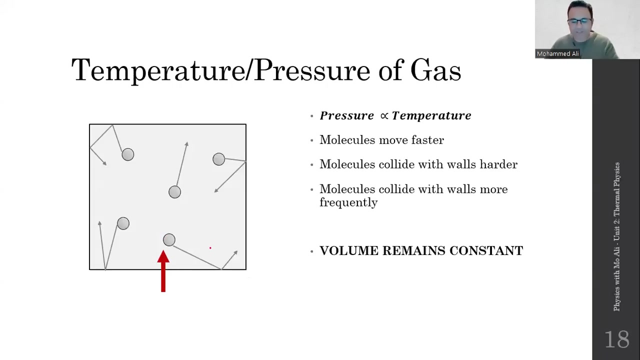 physics? yeah, let's see how gases behave, let's say when heated or when cooled and so on. So how does temperature affect the volume of a gas? We already mentioned that If you heat something like a gas, if you heat something, the molecules move faster and farther apart. 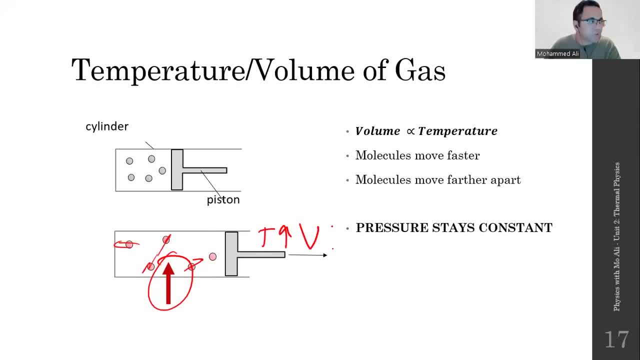 So thermal expansion occurs. So when you increase the temperature, the volume increases. You increase the temperature, the volume increases. Why? Because the molecules move faster and farther apart. So we say that temperature and volume are directly proportioned, which makes sense. 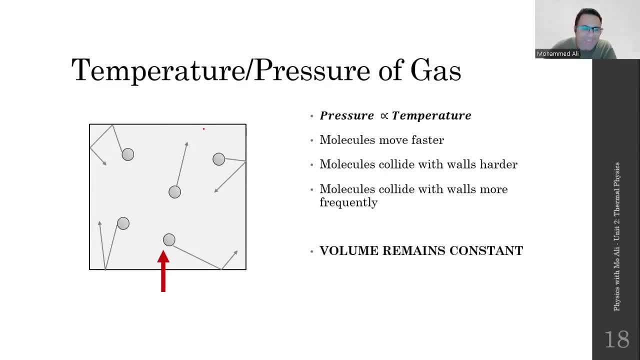 What about pressure If you heat a gas and the volume is constant? you heat a gas and the volume is constant. the molecules, as they're moving faster, they collide harder with the walls of the container, applying more pressure. So when the temperature increases. 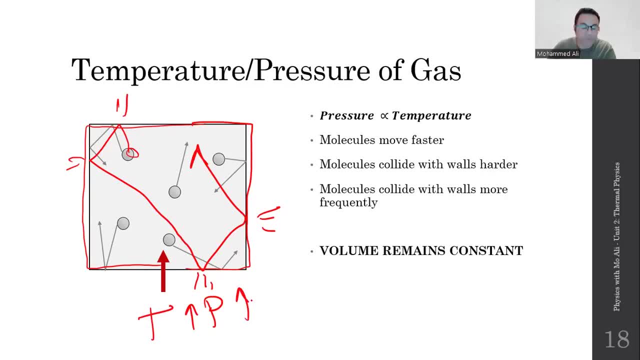 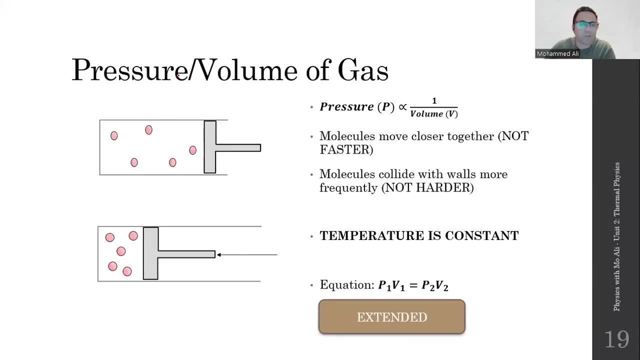 the pressure also increases. So they're directly proportioned, Easy peasy. Finally, how does volume affect pressure? Because here's the thing. but do we have to heat? No, we don't. So when you have a gas inside the piston cylinder arrangement. 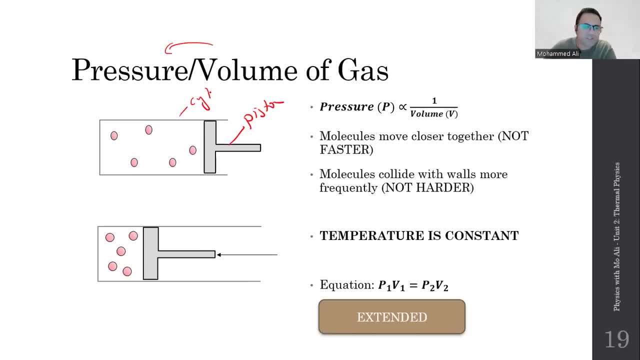 this is called a piston, This is called a cylinder. And you complete the cylinder And you compress it. You forcefully decrease the space between the molecules. And when the space between the molecules decreases, the pressure increases because the molecules are now colliding with the walls. 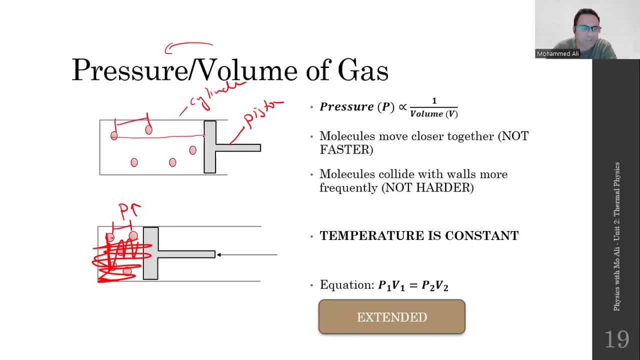 and each other more frequently, Whereas here, because they have a lot, had a lot of free space, they didn't collide with each other as frequently They do now. So when the volume decreases, the pressure increases because the molecules are. 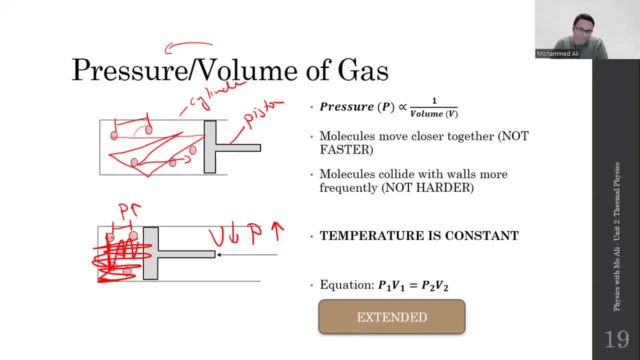 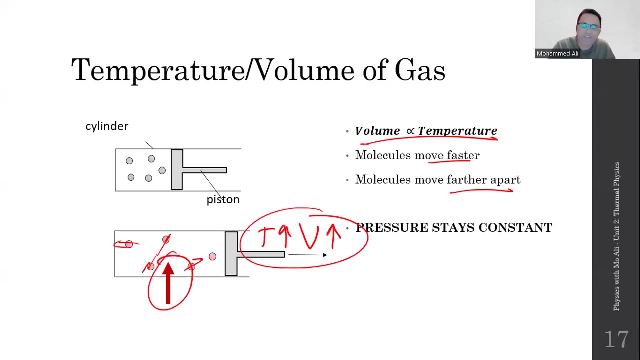 they're colliding with each other more frequently. They're not moving faster, They're not harder, They're just more frequent. Yeah, So we say that pressure and volume are inversely proportional, But wait, there's more. You notice that in every single one of these cases, 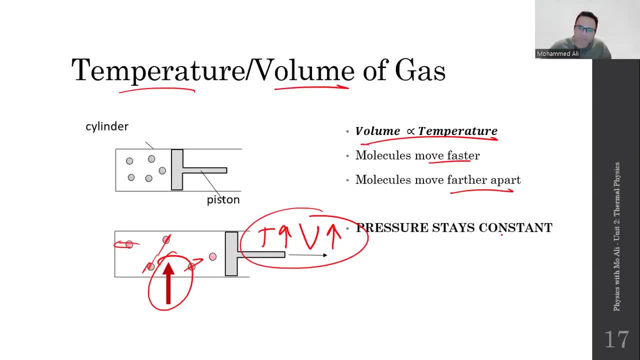 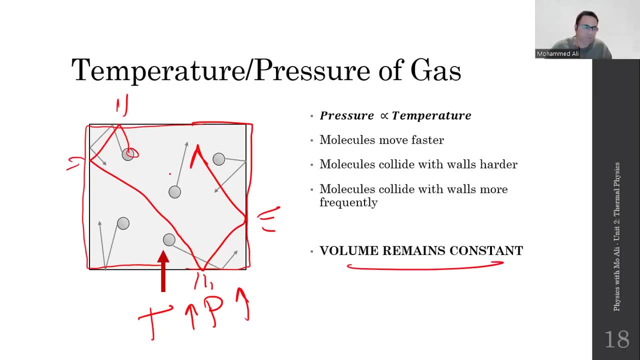 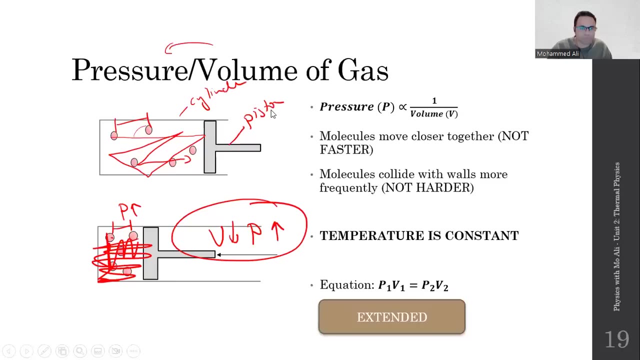 something was constant. If you're heating and the volume rises, the pressure does not change. If you're heating but the volume is constant, like you've trapped it in a container, pressure will increase, Maybe even go boom. And finally, by the way, 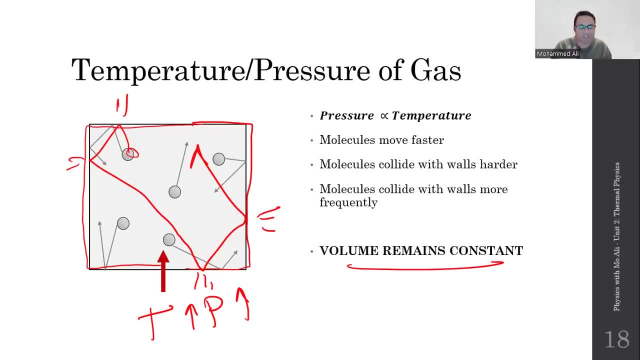 that's what happened with gas tanks in movies When they fire a pistol and it explodes. the reason it explodes is because the temperature of the gas inside increases so much that the pressure of the gas cannot be held in place. with that, can that cylinder? 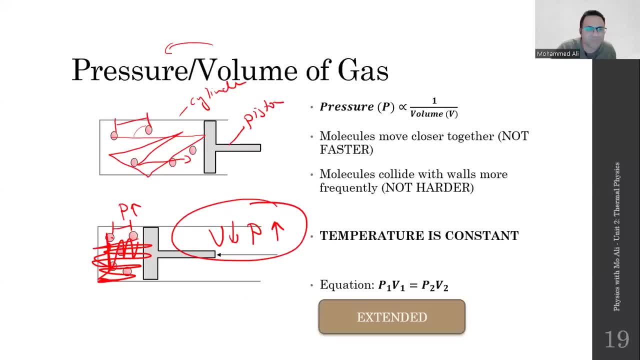 So the cylinder itself blows up because it can't handle the pressure. And finally, when it comes to how volume affects pressure, the temperature was constant, so that's not too hard to achieve, but there's an equation And, as you saw earlier, it's PV equals constant. 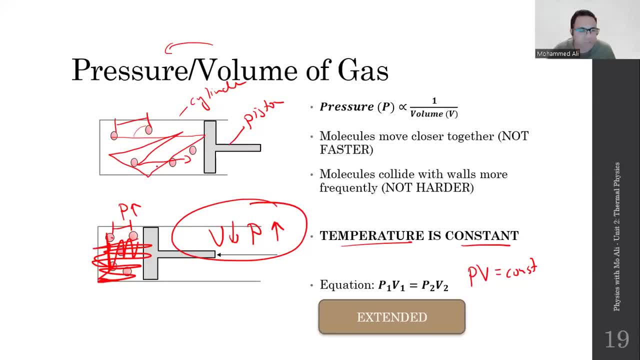 meaning pressure times volume is always constant. So the equation we use is: P1, V1 equals P2, V2, which is the pressure times volume before you compress or do whatever equals the pressure times volume. There's volume after. It's an equation. 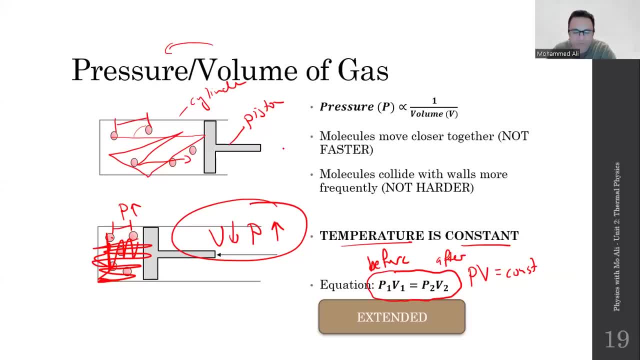 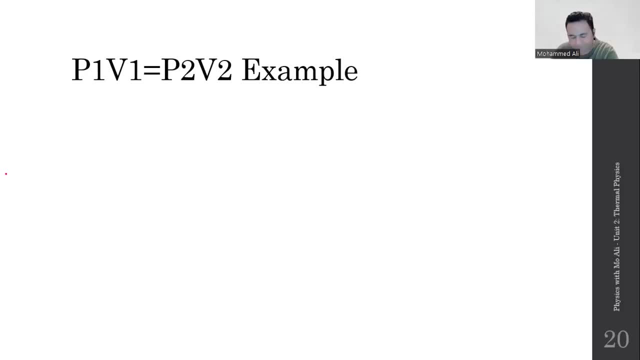 It's a law. So let's see how we do we use this. Let's assume- let's just assume- that you have a balloon. Where's my silence? Oh, there it is. You have a balloon. Let's say the volume of this balloon is 100 centimeter cubed. 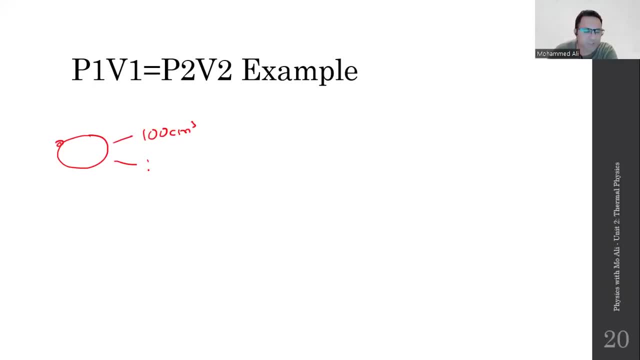 It's not a very large balloon And it has a pressure right now of one times 10 to the power of five Pascal normal atmosphere. But somebody decides to sit on the balloon, So they're going to squish it. Mostly bad idea, but they're going to squish it. 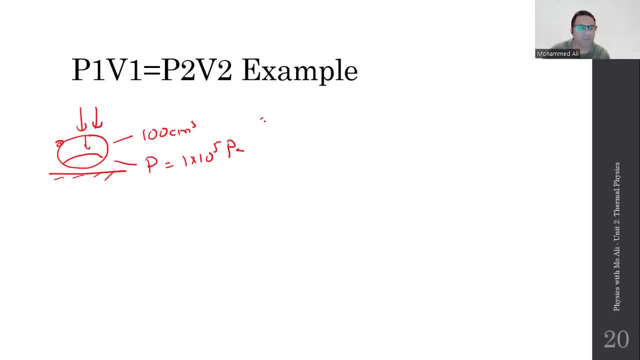 If I tell you that the volume now after the squish is, you've lost how much? let's say, let's say it's 80 centimeter cubed, The volume decreases to 80.. Can you find the new pressure? Of course you can. 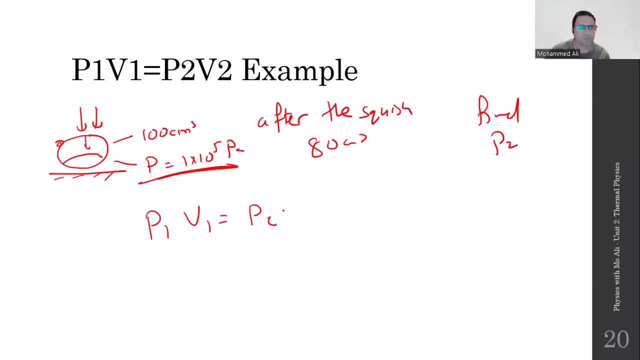 So here's the P1, P1 equals P2, P2.. What's P1? one times 10 to the power of five? What's V1? A hundred? Now you might be thinking: why am I using centimeters in a question which often involves just meters? 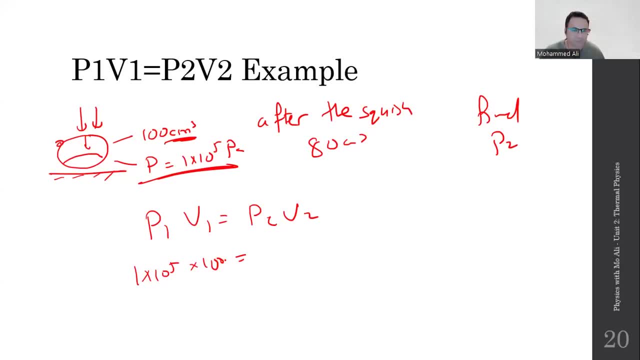 and Pascals and stuff. Just leave it as is. you'll now you'll learn a bit. Let's see what I'm doing. Okay, So pressure one, volume one. no, this is extended, As I said in the previous page, right? 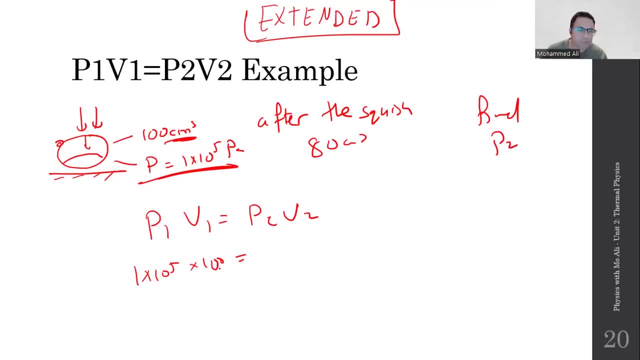 Equals pressure two, volume two. So pressure one is one time 10 to the power of five. Volume was a hundred, No problem. equals what's pressure two? You don't know, I want it times. what's the second volume of the balloon after the squish? 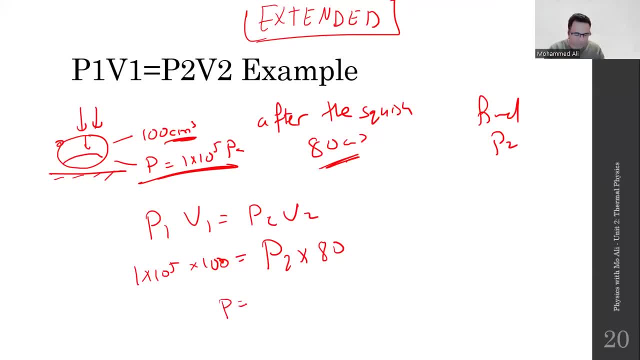 It's 80.. So P2 equals P2.. So P2 is equal to one times 10 to the power five times a hundred, Oops, 10 to the power five times a hundred over eight. This will give me- and I prefer to write my answers. 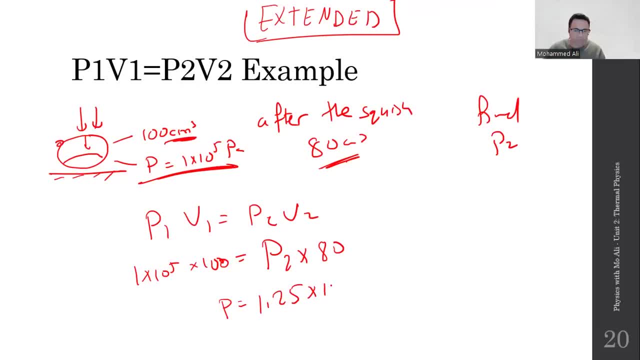 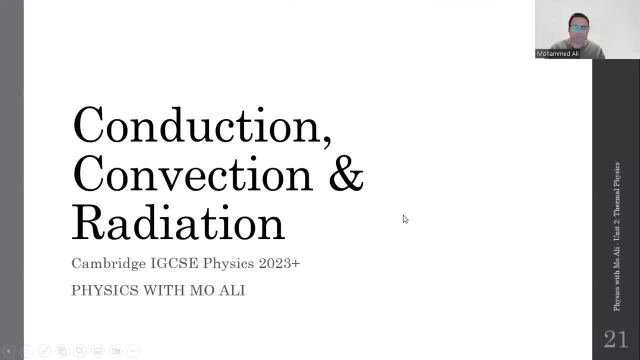 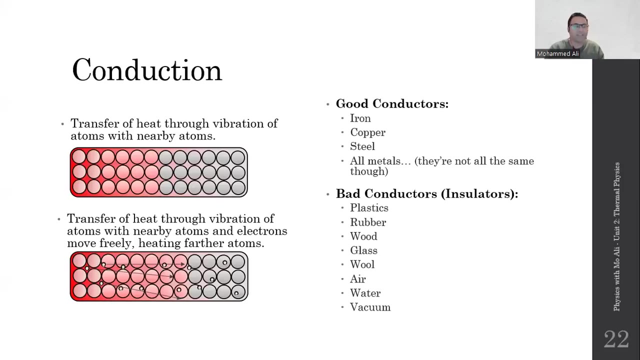 in standard form is. it's very long, 1.25 times 10, to the power of five Pascal. Okay, Done. Next let's move along. Let's talk about conduction, convection and radiation. These are the three methods of heat energy transfer. 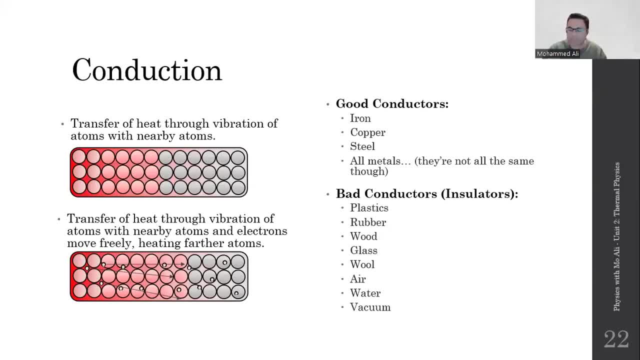 that we have, depending on whether that substance that's transferring the heat is a solid or a liquid or a gas. It's a solid or a liquid or a gas. If it's a solid and you heat up one end of it, here's the sequence that happens. 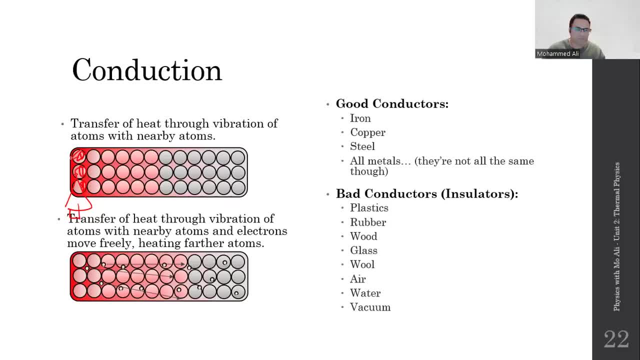 These molecules gain energy, They move faster, They collide with their neighboring energy. So as they collide, they give them some energy and they move faster and that continues to happen. The atoms start to vibrate faster, colliding with nearby atoms. So it takes a long, long time. 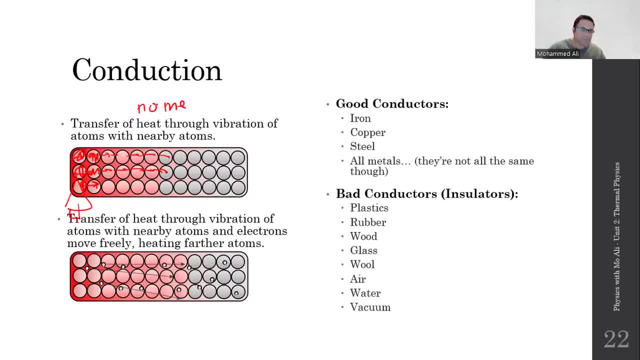 This is how conduction occurs in non-metals, by the way. What about metals Now? unlike non-metals, metals also have what we call free-moving electrons. free-moving electrons, So you've got double the conduction capacity, or more. 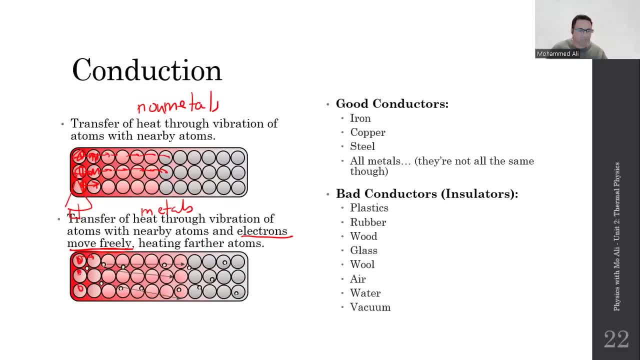 because the atoms sure, they gain energy and they vibrate and collide with nearby atoms. But then you've got a lot of free-moving electrons. As soon as they gain heat, what do they do? They travel very quickly, Quickly through the solid, reaching the farther ends. 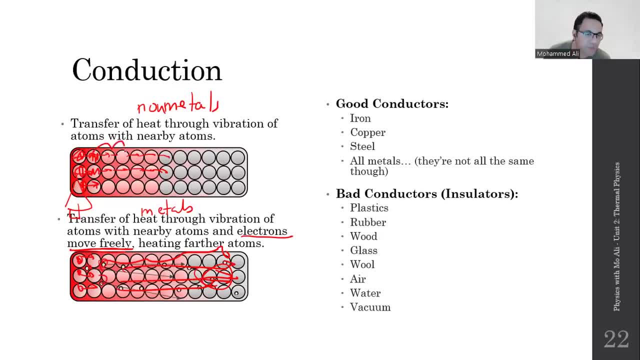 and colliding with atoms at the farther end, Not just nearby atoms, No, they collide with everything along the way. That's why metals are such good conductors of heat. Why are they good conductors of heat? Because they have free-moving electrons. 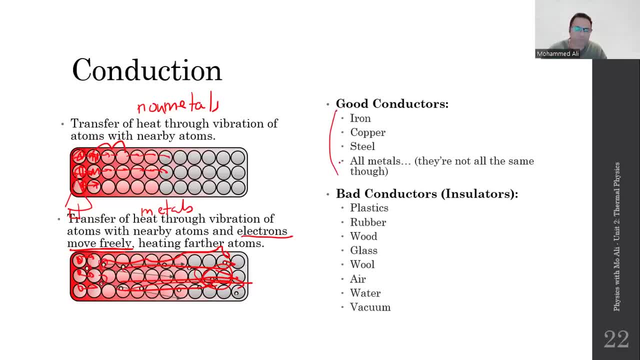 So examples of good conductors: basically all metals- iron, copper, steel. keep them in mind if you're ever asked to suggest a metal. What's a bad conductor? Anything that you know: Plastic, rubber, wood, glass, wool, air. 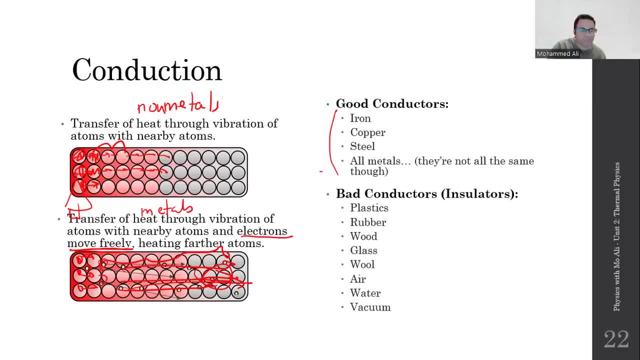 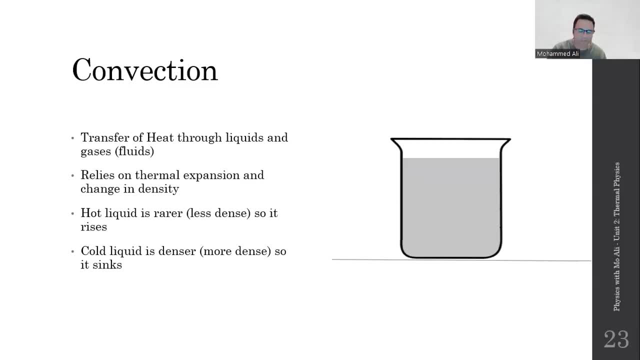 Very good. So that's the difference in conduction between a non-metal and a metal. What's convection? Very important because it's often required to be described properly. So what is it? So it's when heat can travel through the metal. 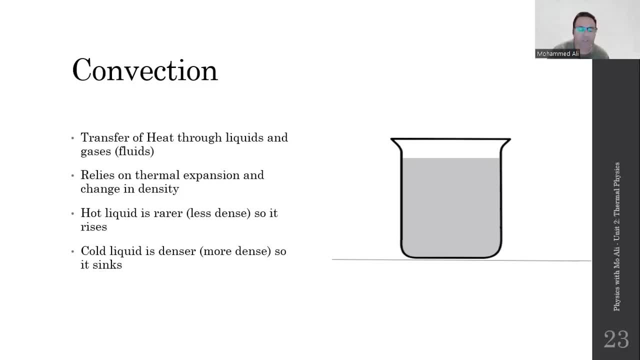 Heat can travel through a liquid. Heat cannot travel through a liquid by conduction. You might be wondering why? Well, that's because molecules and liquids slide over each other. They don't collide with each other very frequently. So instead, what you do is: well, if you heat this corner. 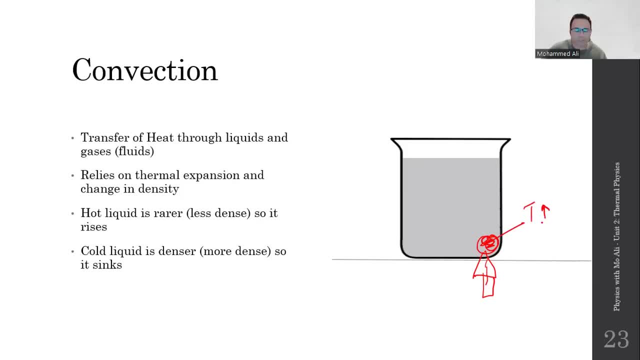 what's going to happen to the liquid here? You'll say it gets hot. Okay, So when it gets hot, what happens to its volume? It increases, it expands. And when the volume increases- this is the important bit- The density of the liquid decreases. 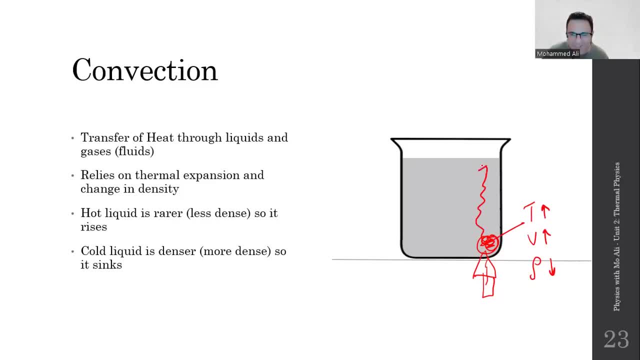 It becomes less dense. And if a liquid is less dense, it will rise and it will float. Okay, cool, You've got hot water that goes up. What about the cold water? that was already here? It goes down. So you've got hot water rising and cold water sinking, all right. 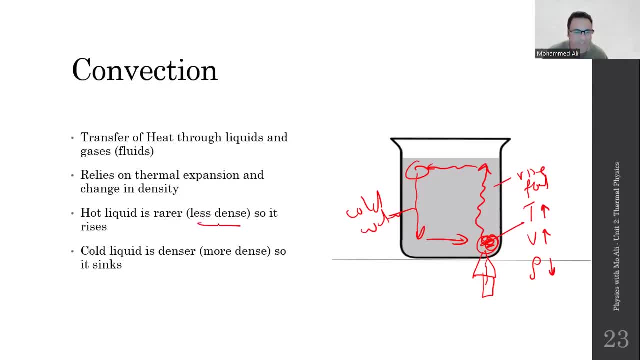 Why? Because hot gases are less dense, Cold is more dense. This cycle is called the convection correct. This cycle is called the convention Convection. Convection, Convection is the current. There we go. So remember it doesn't only happen in liquids. 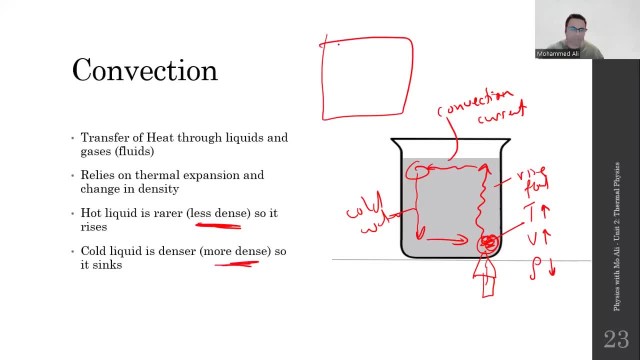 It also happens in gases. So if I have a room and I have an air conditioner in the room, in this corner of the room, if I cool down the air, cold air sinks because it's more dense. hot air rises because it's less dense. 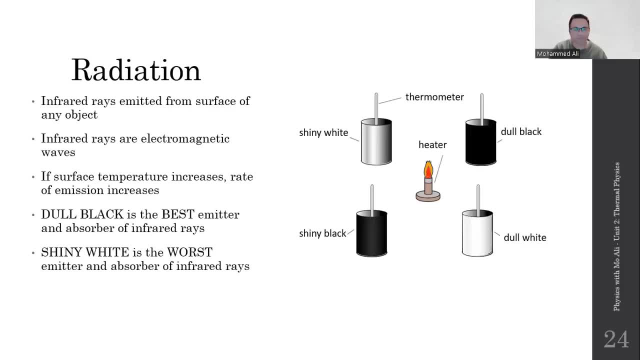 Radiation The last of the three, The three methods of heat transfer. Radiation is basically an infrared wave emitted from the surface of any object as long as it's hot. If an object has temperature, which means everything, it emits an invisible type of wave called an infrared wave. 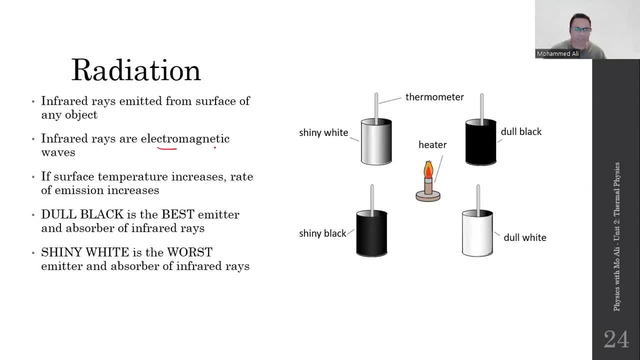 which transfers heat. Now, infrared waves are electromagnetic. They're released from the surface of the object. But what does it depend on? Like what's it's affected by? Obviously, obviously, temperature affects it. If you heat it, it's going to be hot. 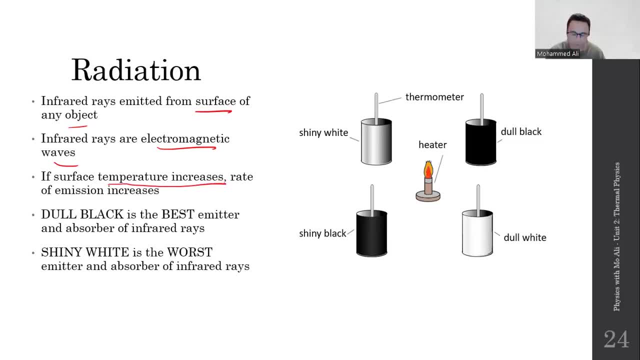 If you heat something more, it will emit more radiation. All right, What else does it depend on? And that's very well. second, it depends on size. If you have two objects, one that's small, one that's large- 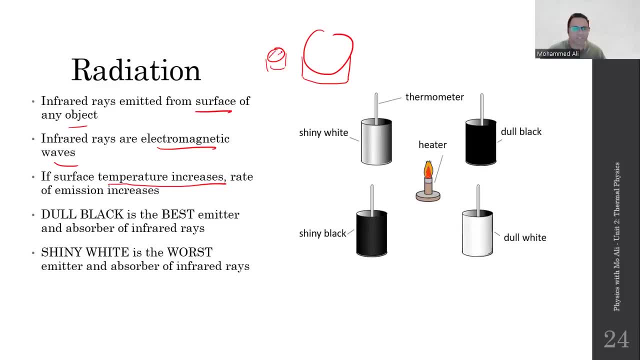 and they both have the base. Basically, this is their surface area. The large one would be always best for radiation. Why? Because it's a larger surface area, So there's more of the hot surface that gives out heat. All right. 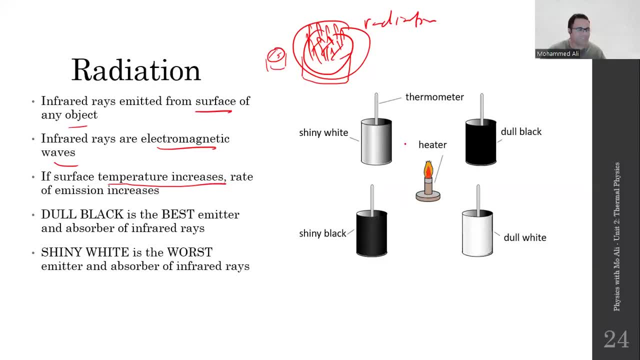 The third thing that affects the third thing that- I'm sorry, somebody sent me a funny joke- Third thing that affects how much heat is absorbed or emitted by a surface is the color. This is the most important bit. We say that black is the best emitter and absorber of radiation. 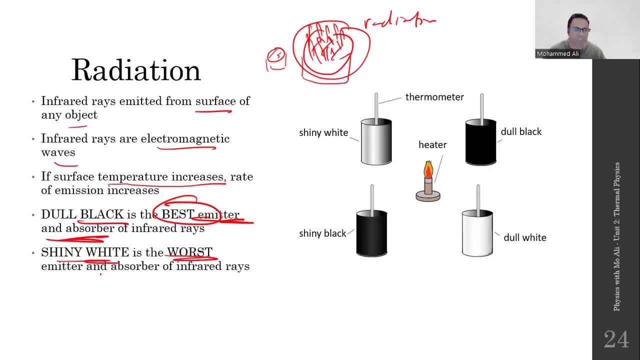 We say that black is the best emitter and absorber of radiation Or infrared waves, Whereas white is the worst emitter and absorber of infrared radiation. Now, what do I mean If I get you these four cans, as you can see? 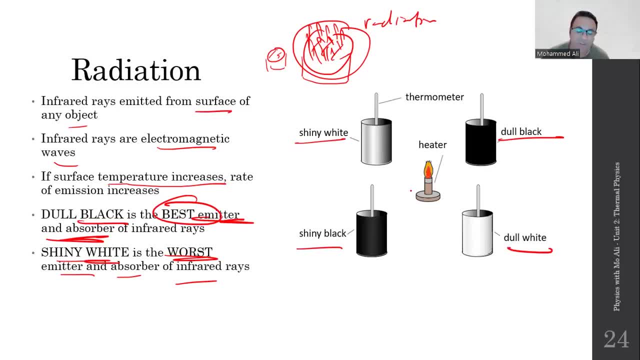 one of them is dull black, one of them is shiny white, one is shiny black and the other is dull white. And you put a heater between them, all three of these will get the exact same heat. the same time You will realize that the black will give you. 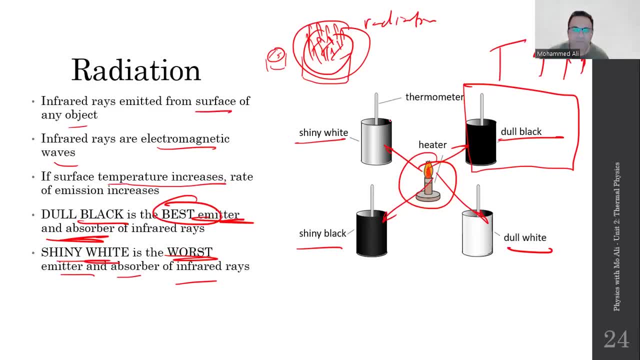 the highest temperature increase, Whereas the shiny white or the silver will give you the lowest temperature increase. All right, So black is the best absorber. It's very easy to absorb. Shiny white, because it's a good reflector, is not a very good absorber. 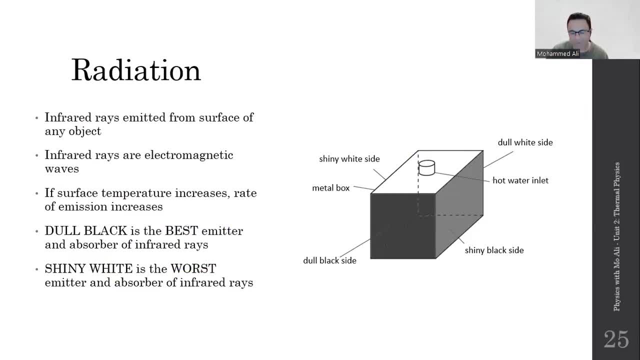 They're also the best emitter and worst emitter, black and white respectively. If you get a container and you pour it full of hot water, this means that all of the surfaces are at the same temperature, so they should be emitting heat at the same rate. 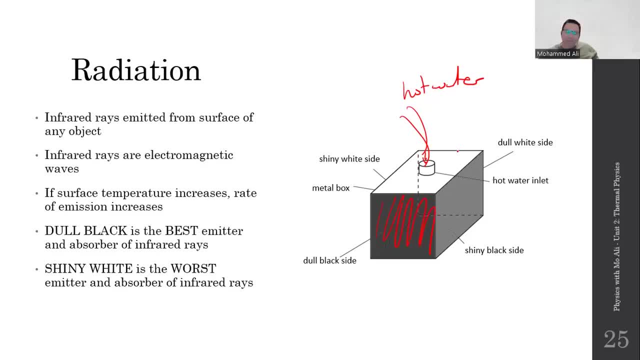 But no, if you paint each face of that box a different color: one's dull black, the other is shiny black, third is a is dull white, and the fourth is what Shiny white, The shiny white side, will emit. 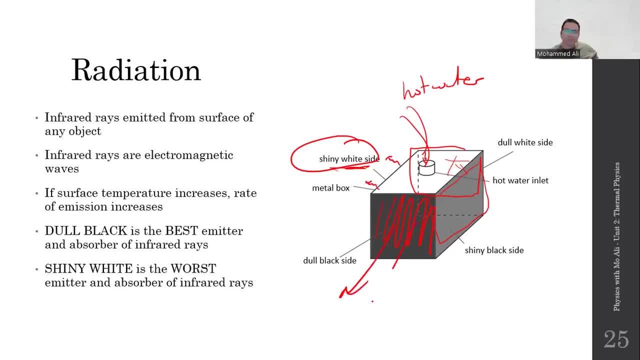 because now the object is hot, the least amount of radiation, Whereas the dull black side will emit the most amount of radiation. So remember, black is the best in both of the cases. So I love wearing black, but in both cases best emitter and best absorber. 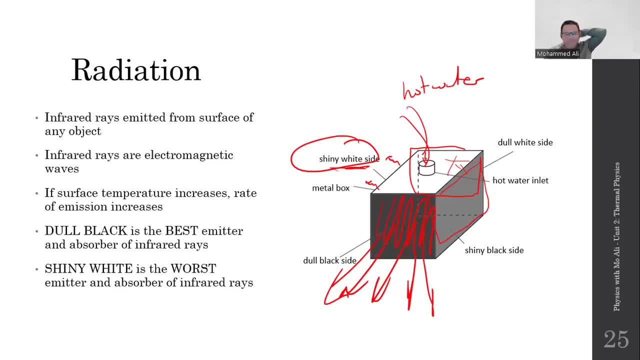 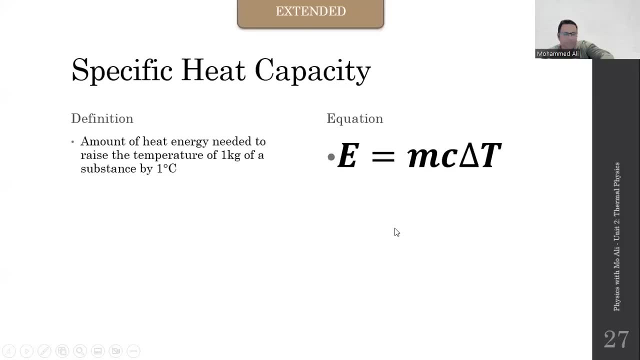 Silver is the worst emitter and best absorber. Silver and absorber Shiny white- is silver essentially. Yeah, The last thing we want to discuss for today- and we'll end the session after we're done here- would be specific heat capacity. 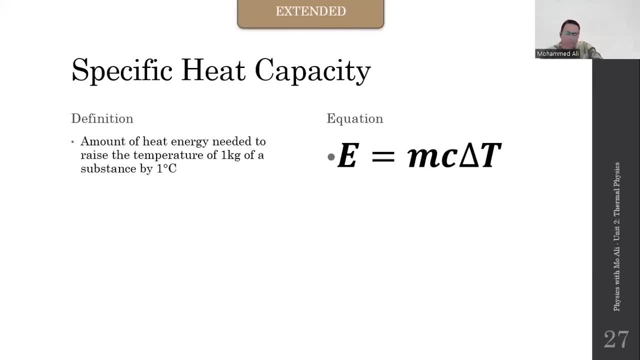 What do I mean by that? If I give you a bottle of water and I ask you to go ahead and heat it, you'll just pour it into a kettle, for example, and turn on the switch or put it on a stove top. 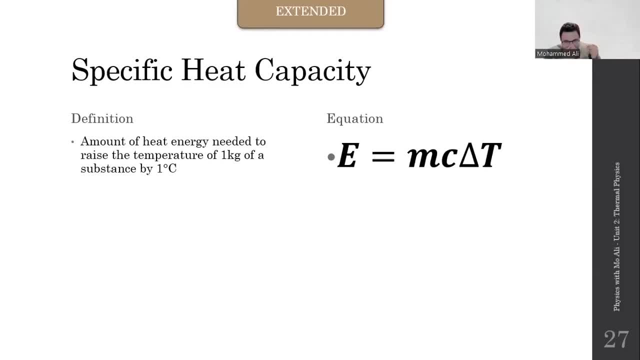 like, if it's not a digital kettle. So as the water heats up, it needs energy to keep heating. The question is: how much energy? how much energy do we need? Well, that depends on a few things. First, it depends on the mass of the substance. 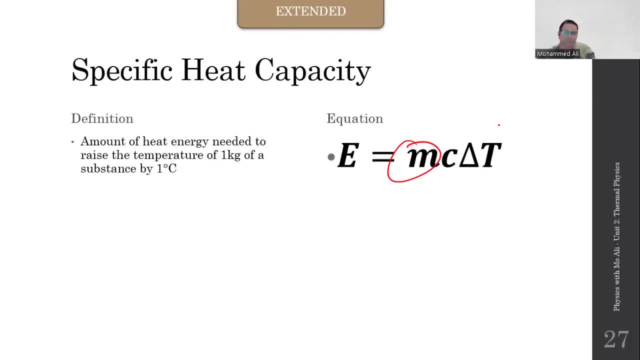 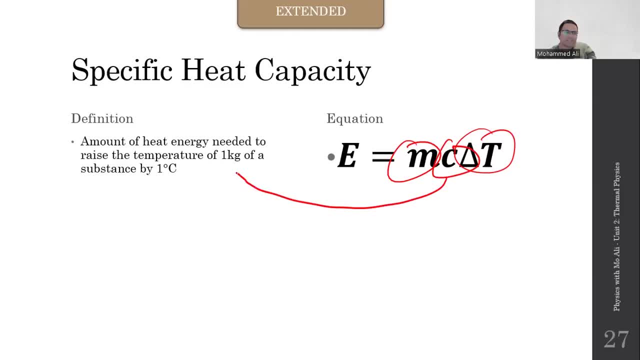 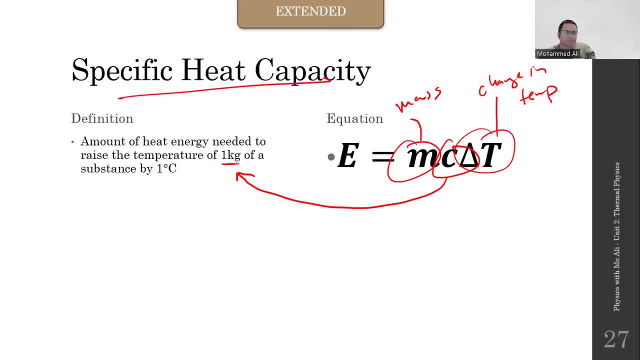 which is the amount of heat energy needed to raise the temperature of one kilogram by one degree Celsius. This means that if I have one kilogram of, let's say, water- because it's a very common substance- water, I can tell you that in order to heat it from 20 degrees, 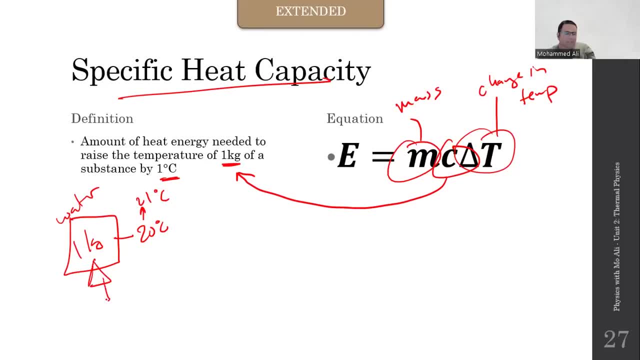 to 21 degrees, I need to give it 4,000 joules, for example. This is called specific heat capacity. It tells you how much energy does that one kilogram of water need to be raised by one degree Celsius? That's all you need. 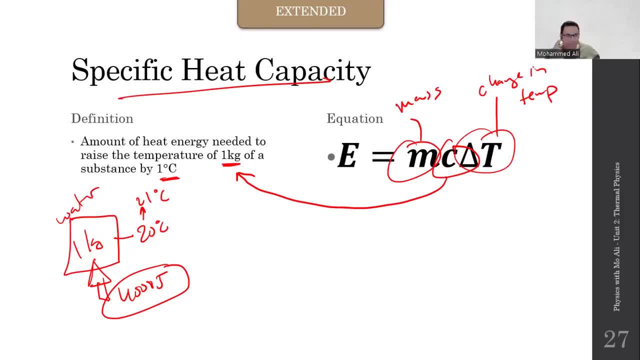 That's all it is. How much energy does one kilogram need to be raised by one degree? If I want to raise it by 10 degree, you multiply it by the change in temperature. If you want to find out what if you had less. 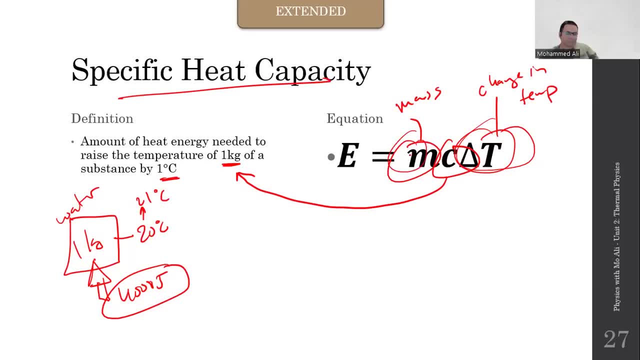 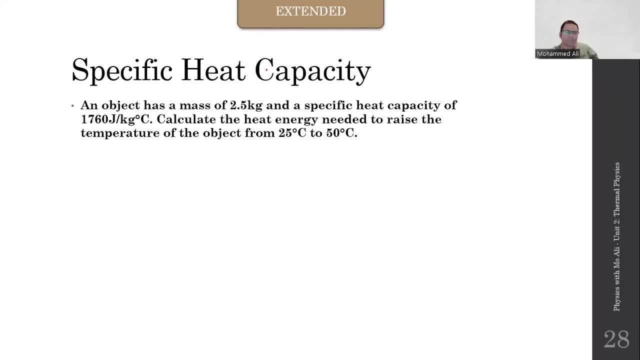 than one kilogram. you multiply it by the mass, It'd be half a kilogram, it could be a quarter, whatever it is, Now let's see how we can use this. for me, An object has a mass of 2.5 kilograms. 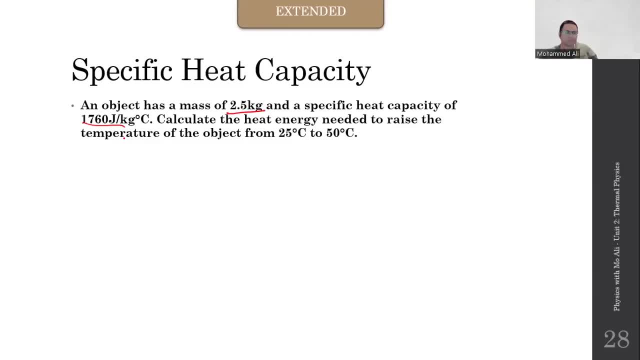 and a specific heat capacity of 1,760 joules per kilogram Celsius. So he's giving me the mass and he's giving me the specific heat capacity. Calculate the heat energy needed to raise the temperature of an object from 25 to. 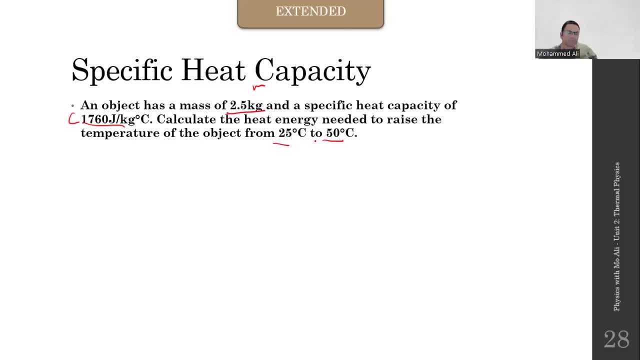 25 to 50.. 25 to a 50., 25.. So calculate the heat energy. E equals MC, delta T. What's M 2.5.. What's C 1,760.. And what's delta T? 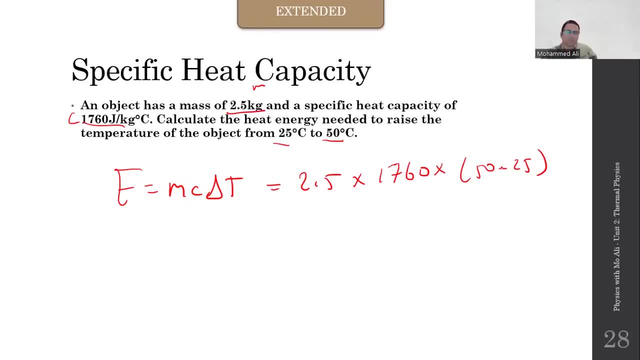 50 minus 25.. Because I want to change, in this case the change in temperature, The 2.5 times 1,760 times 50 minus 25.. This gives me a nice answer of 1.1.. Oh times 10 to the power of five. 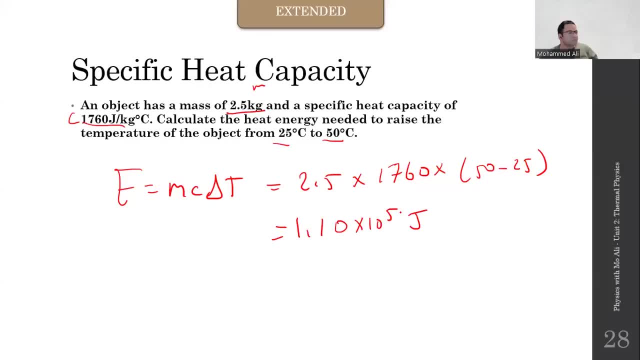 Do you have any questions regarding specific capacity or anything before that? Oh, I see a question. Is the radiation only infrared waves that are emitted or absorbed? Yes, The black and white that we're talking about would be just radiation. And can you repeat how to calculate the pressure of a gas? 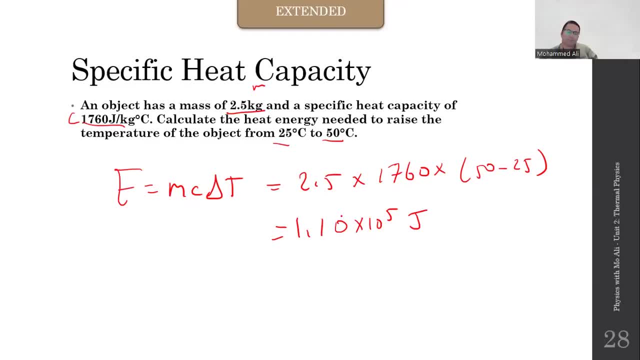 Of course, I can go back and show you how again, but let's stay here. This: what does the C stand for? The C stands for specific heat capacity. All right, Excellent, You got it. Excellent, You're welcome.